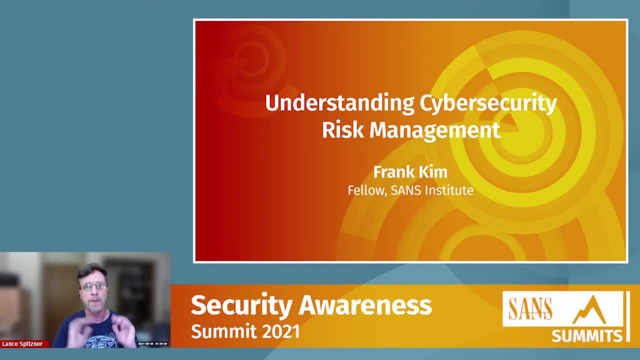 leadership's language. You are now aligning your program with their priorities And you're going to have a whole lot more budget, a lot more credibility And, to be honest, this is how you go from security awareness officer to, if you want it, to, becoming the chief information security. 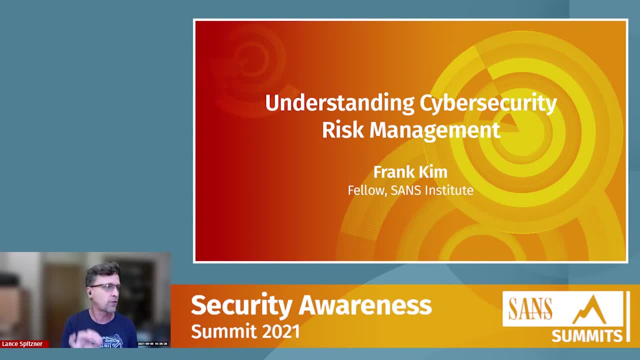 officer. This will open so many doors for you in so many different ways And, like I said, the reason I'm so excited to have Frank join us is not only has he been a CISA and he's been in these situations, not only is he one of Sam's most 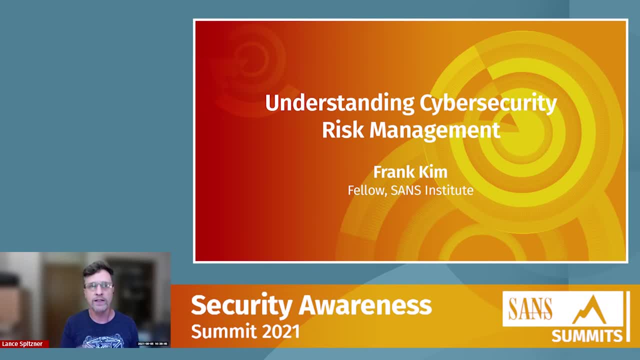 Uh-oh, CISA Senior instructors. But he has written several Sam's courses on how to do what we have just been talking about all day long. So in just a moment I'm going to turn it over to Frank And, like I, 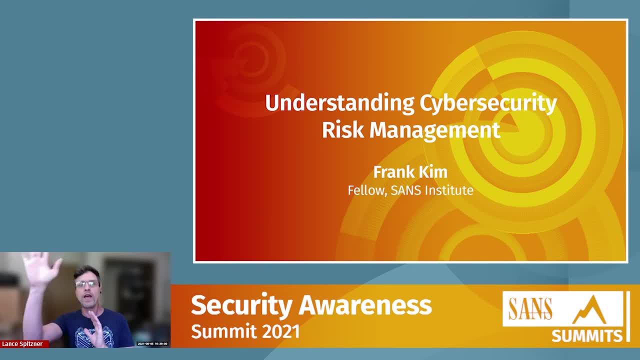 said, though, if you're already experienced with this, head over to track two and learn about security culture from Janan Baj. If you're not familiar with this, you're in for a treat, because it's going to be a very simple, nice introduction to what this field. 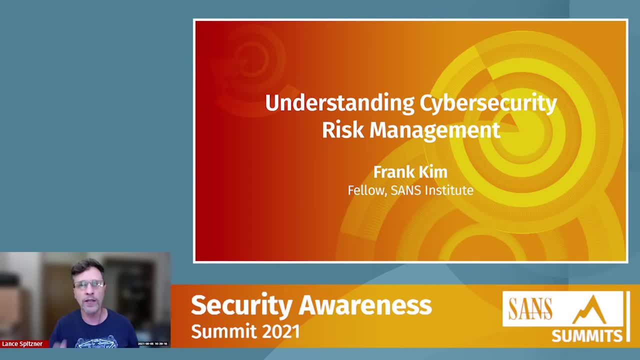 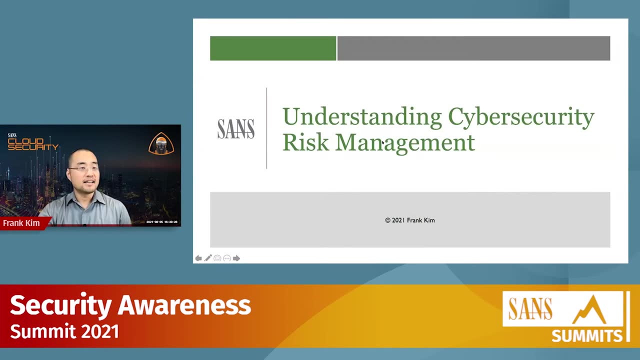 is and why you should care. All right, I've been talking enough, Frank, enlighten us with your great expertise. Hey, thanks so much. Hey, I realized that I didn't change my background from a prior meeting here, but we will just leave it the way that. it is Sorry about that, folks. So, hey, thanks so much. 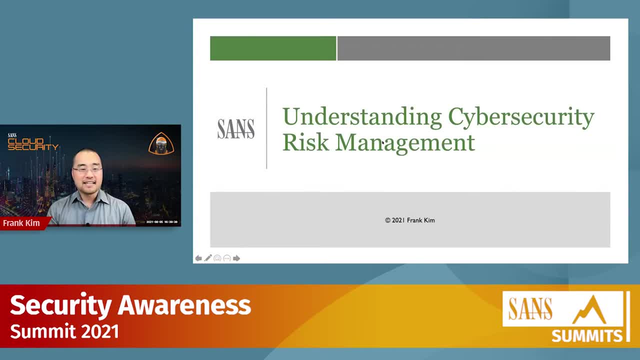 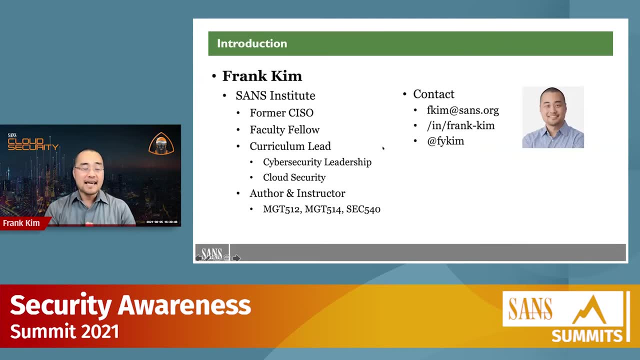 for the kind introduction. Lance Really appreciate it. Let's go ahead and dive right in here to understanding cybersecurity risk management. Now, as Lance mentioned, my name is Frank Kim. I've been teaching writing courses with Sam's for about 14 years now. I currently lead our cloud security curriculum and our cybersecurity. 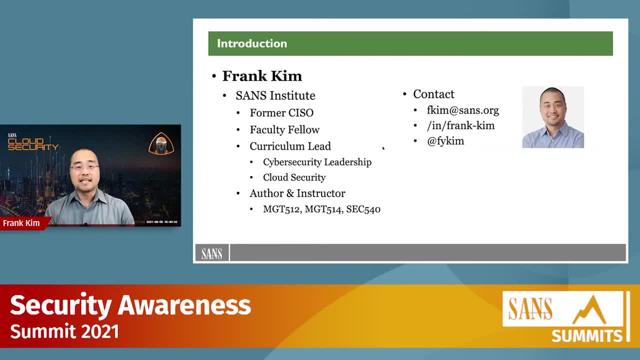 leadership curriculum, of which this topic, as Lance was mentioning, is an important part. If you want to reach out, contact me at any time after this talk. During the talk, of course, you can feel free to go ahead and chime in with Slack, you know, throw those proverbial tomatoes. 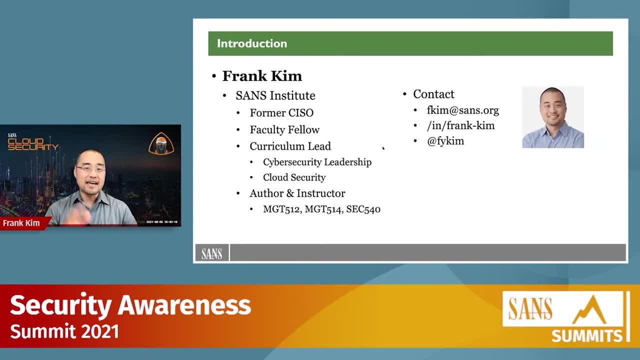 if you will. I am watching Slack here right at my eyeline, So any comments that you post here I will get to them pretty quickly. But after the fact, if you want to reach out and continue the conversation, feel free to email me, hit me up on social media and so on. All right With that. 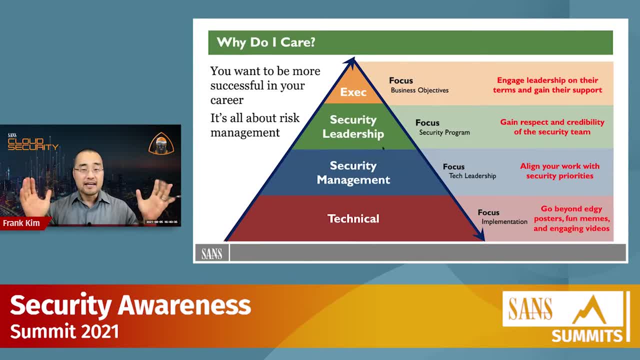 being said, let's go ahead and dive right in. You know we've got a summit full of security professionals, security awareness professionals, awareness officers, and so on. So the question that we always like to start with is: why? Why do we care? Why do you care? Why do you want to be here and listen to this specific talk? 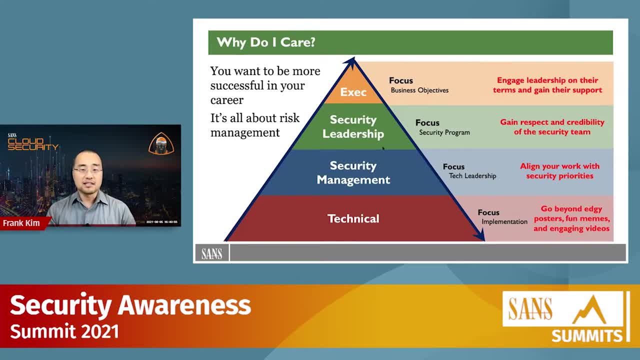 Now, certainly we all want to make our organizations a little bit more secure. We all want to improve the state of our businesses. We all want to do the right thing, And one of the other reasons that many of us are here toiling away in our careers is that, yeah, well, we want. 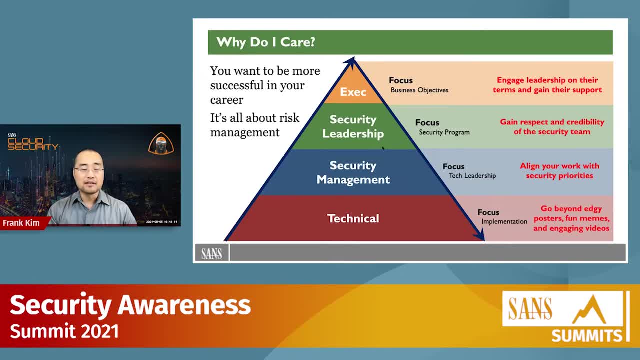 to be more successful, And to be more successful, it's all about risk management Now. I started my career over 20 years ago as an engineer, as a developer, building applications, building systems and deploying fun and cool new technologies. Now I would sit at my for the first. 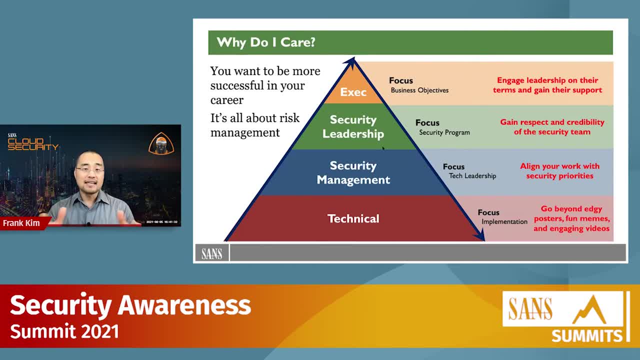 many years of my career, I would largely sit at my desk, sit at my cubicle on my own, and I was happy right Typing away, writing code, deploying various things. I was really focused on the technical layer of this leadership pyramid that we see here on the slide. 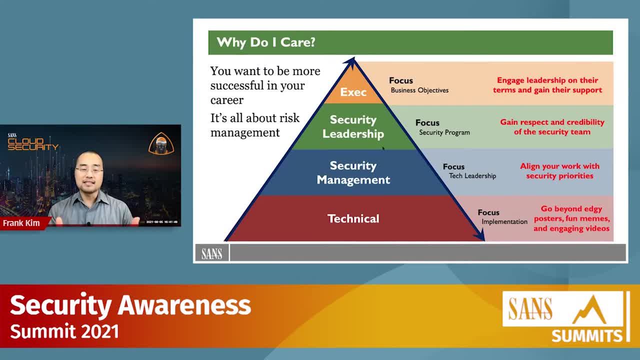 As I progressed in my career, I realized you know what. It's not just about that technical foundation that is, yes, very useful to have in place. It's about, well, how do you lead and influence other people, And so I got a little bit more interested in technology leadership. 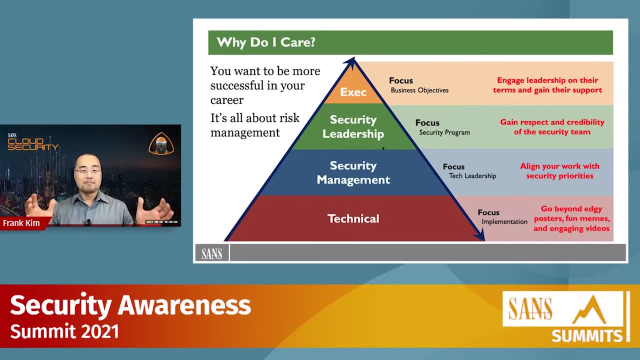 But then from there it was okay. well, how do we take a step back and think about this as a program overall that ultimately, at the top of this leadership pyramid, is helping your organization achieve various business objectives, Whether that might be a customer-focused mission, whether that might be a financially 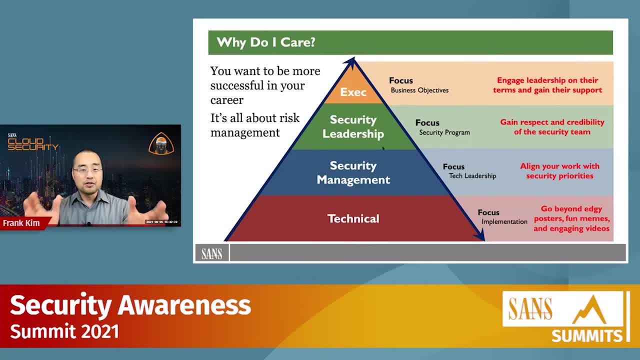 driven mission. Now for us, for you, as security awareness professionals. what does that mean On the right-hand side, here in the lower right-hand corner, as Lance was just pointing out? Now, one of the fun things, one of the cool things that security awareness does is- I liken it to the 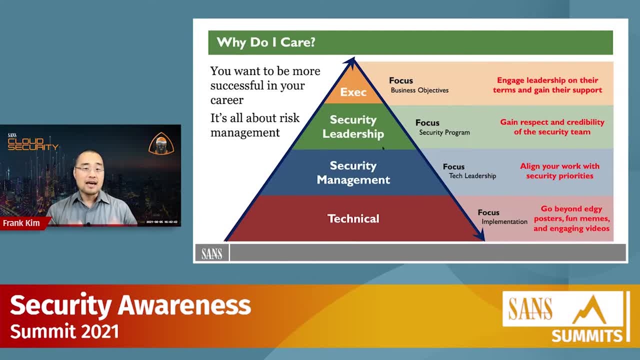 various technical activities that I was doing as an engineer at the very beginning of my career and throughout, Doing things like Marketing, effective communications, those edgy posters, fun memes, those engaging videos. We have to have all of those things, But as we progress we want to make a little bit more of an impact. 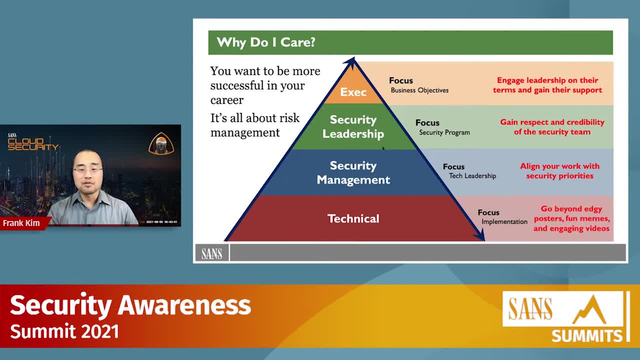 How do we do that? Well, security awareness, overall cybersecurity program. we need to understand what technology leadership cares about: aligning our work, your work in awareness, with those of the other larger security priorities and ultimately gaining respect and credibility of the security. 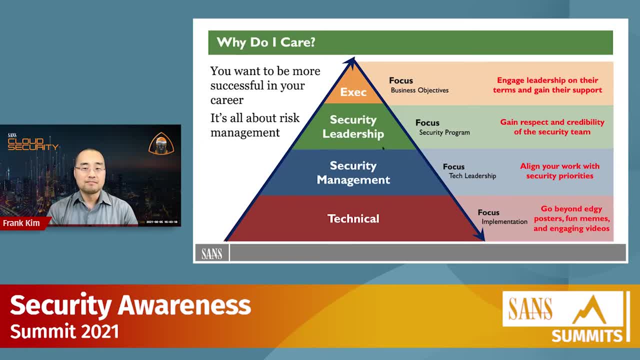 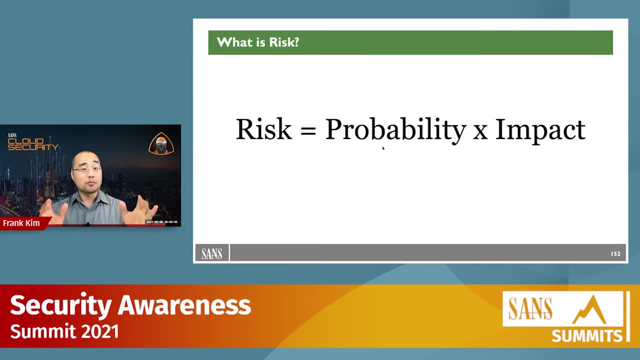 team to Ultimately at the very top right hand corner, gaining leadership's overall support as well. How do we go about doing this? As Lance said, what we're going to talk about is the very basic risk calculation here. This serves as the foundation for everything that we do, not only in awareness. 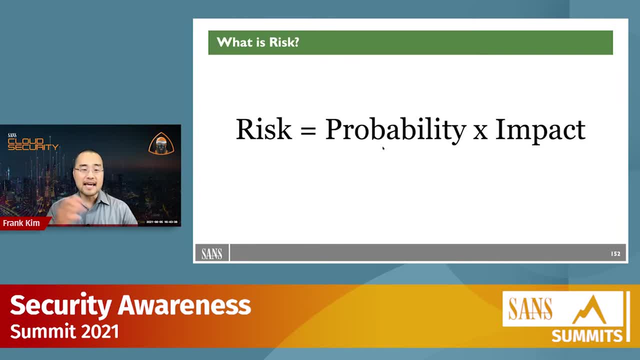 not only in cybersecurity, but a lot of what we do in our day-to-day living here. Reminder: what is risk? Really? risk is just Probability. Time of day: Um, impact, right. Impact- what is the bad thing that can occur? Probability- what is the likelihood that? 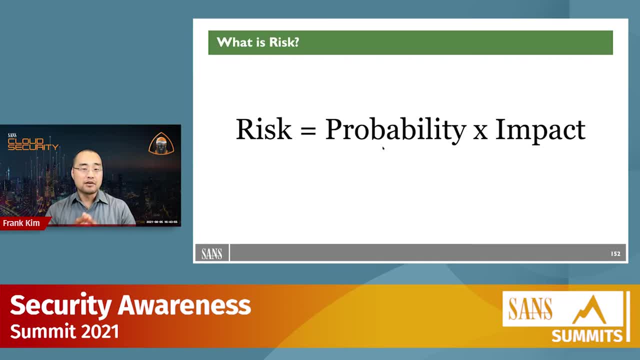 that is going to happen. It is the combination of both of those things: that where we want to try to better understand risk for ourselves, risk for our organizations. Now I'm going to switch to the next slide here momentarily, And this next slide is just an image. that is the best graphic that I. 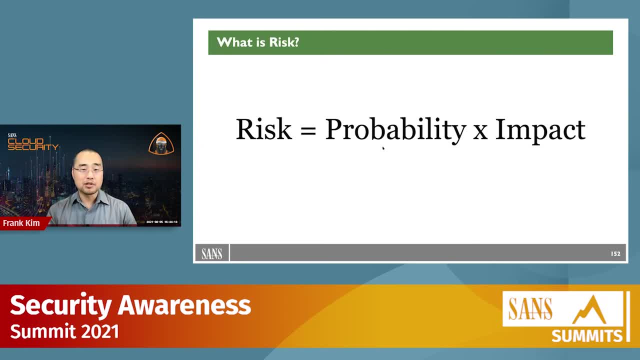 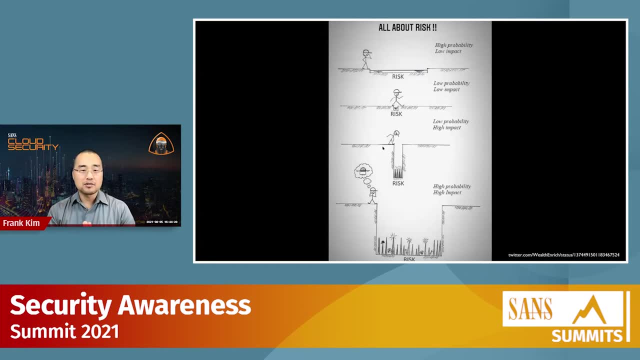 have seen depicting, explaining in simple terms what risk actually is, And if some of you may have seen this online, this was making the rounds on Twitter social media not too long ago. If we take a look at this, at the very top you've got somebody that is looking to get from point A to 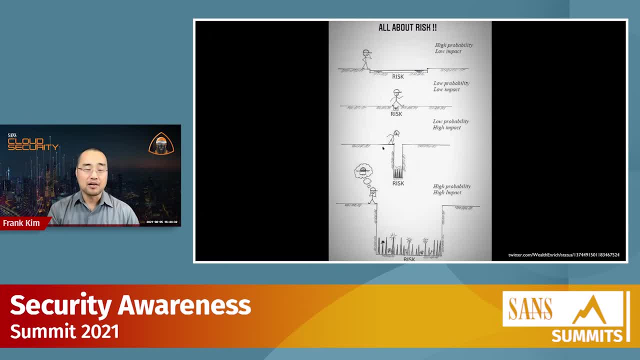 point B. but they want to do it without getting wet, without getting hurt. Well, at the very top you've got high probability that they're going to get wet trying to cross this chasm, if you will, but it is low. 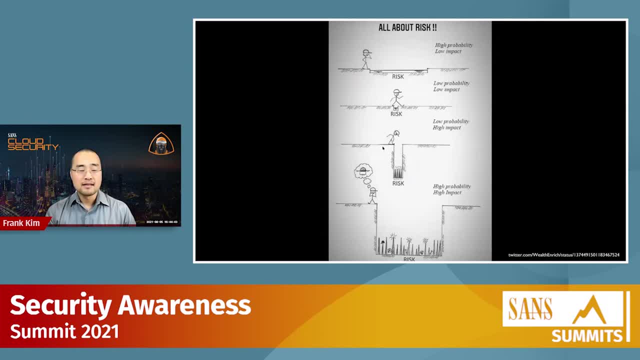 What is the big deal if their sneakers get a little bit wet? The second part of this image here, in terms of low probability, low impact- Well yeah, low probability. you can just step over that little pothole And if you were to, maybe you would twist your ankle just a little. 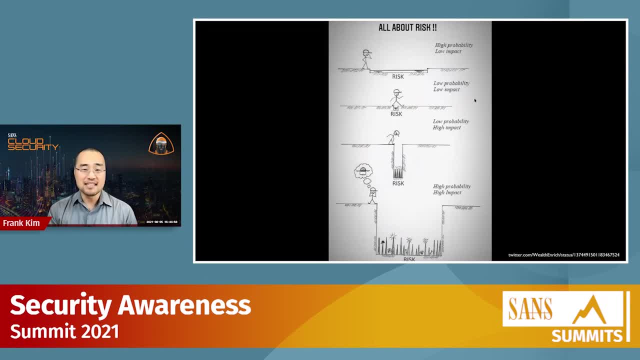 bit, maybe get a little scrape, maybe dirty up your prized Jordan sneakers right? Low probability, low impact, depending on who you talk to. But down below we've got low probability, high impact. Very easy to jump over this little ledge here. 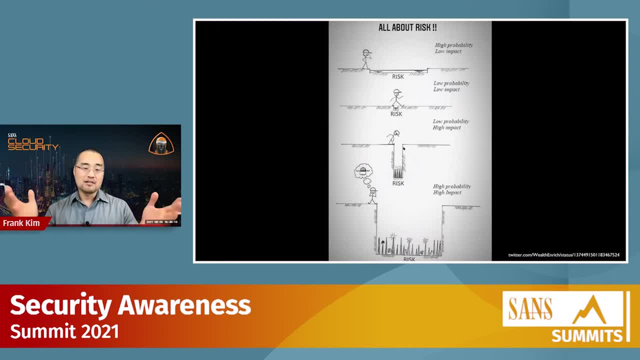 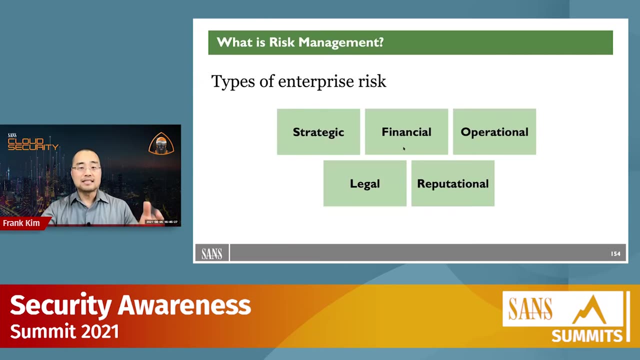 But if you do make a misstep and slip, hey, you could come to serious injury And of course, we've got high probability, high impact down here at the bottom. So why do we talk about this? And we'll circle it back to security here in just a moment- but we need to also understand that this 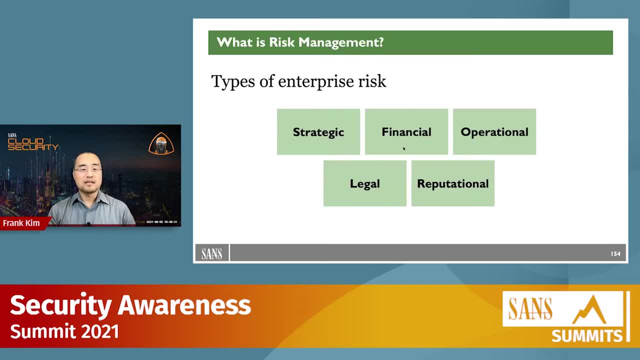 is exactly what our senior leadership is thinking about every single day: Your boards of directors, your board members, your CEO, your CFO, your COO, all of the leaders of the various business units in your organization. They're asking themselves if I make this. 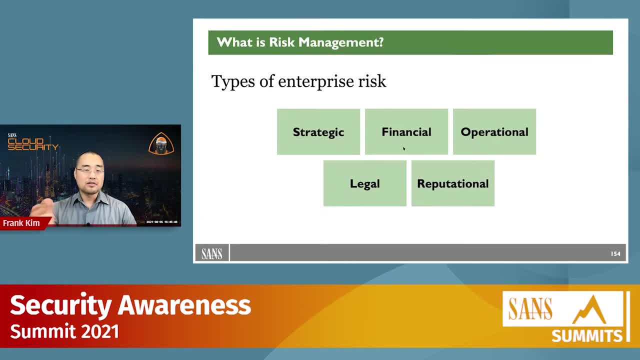 decision. if I decide to cross the proverbial street, what are the chances that I'm going to get hit by a bus? And we need to understand that there are different types of enterprise risk. There is strategic risk. Does the organization want to undertake a certain business activity? 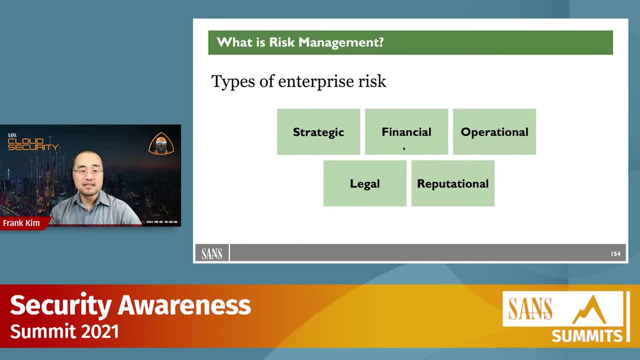 I know some organizations that have purposely decided not to do business in China because they said, hey, from a business perspective we don't want to do business in China, We don't want to take that strategic risk. So engaging in a certain activity or 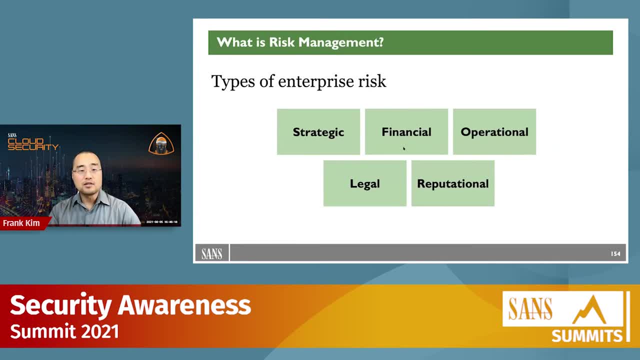 not engaging in a certain activity is a way to manage that element of your enterprise risk, overall Financial risk, of course. How much are we going to lend out? How much reserves do we want to carry? How much should we pay for a certain acquisition? Those are all financial. 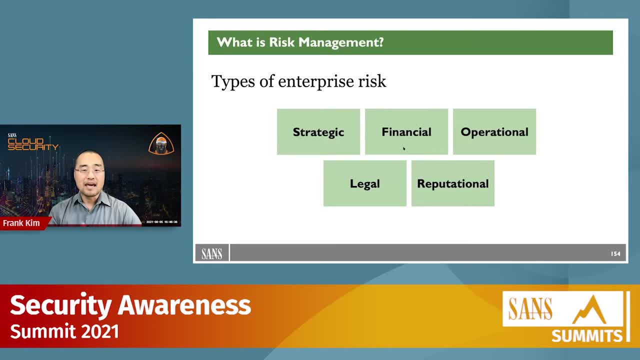 related aspects From an operational perspective. every single day, when you're crossing again that proverbial street, you are making a risk, You're making a risk, You're making a risk, You're making some decisions. Your business is making some decisions on whether or not something is. 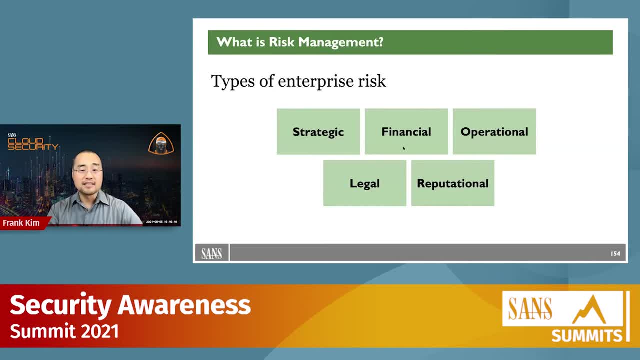 risky or not. Compliance regulatory requirements fall into there, and under the general legal category as well. And then, of course, you've got reputational risk as well. Now do you guys think that? where does cybersecurity come into play of all of this? How come we don't list cybersecurity? 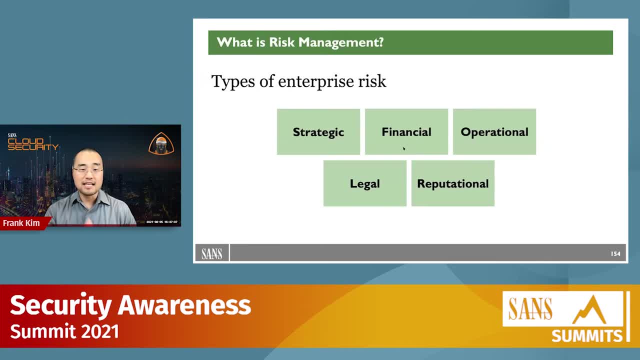 risk here. Do you think that it could crosscut all of these, have an impact on all of these different elements? Do you think that it could crosscut all of these have an impact on all of these different elements? Absolutely, And that's exactly a type of thing that we need to be. 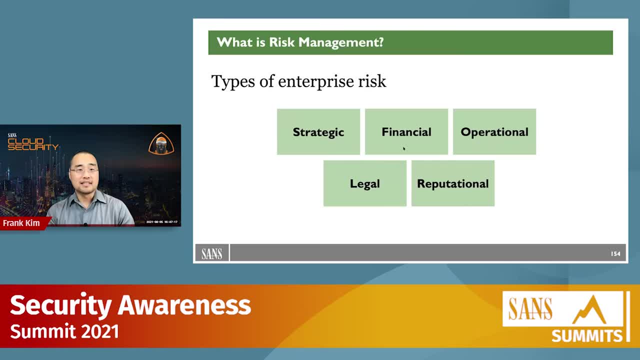 considering. Alan has an extremely excellent point: that risk is also dependent on the size of the organization taking a risk. Do you think that a large financial institution like a JPMorgan Chase when compared to a smaller organization still in financial services, like a small credit union? 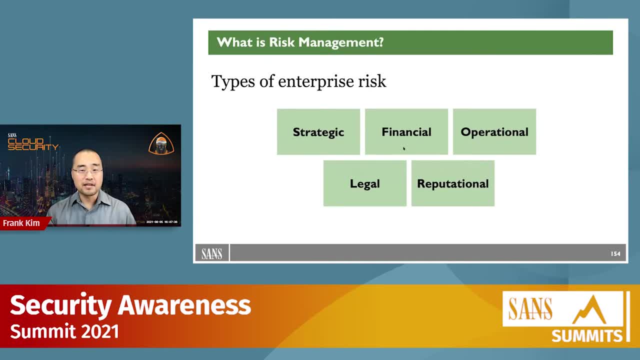 that they've got a much smaller portfolio, much smaller footprint that they're actually managing. So, yeah, that definitely informs The impact portion, the impact portion and the probability portion of the risk equation that we were just talking about. So, excellent point there. Excellent point there, Alan. Now let's break this. 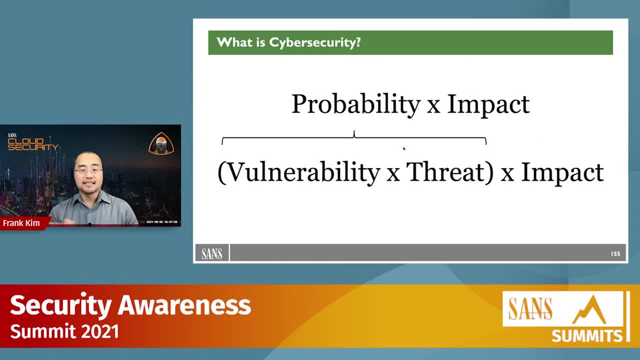 down a little bit more. We already said that risk is probability times impact, But let's zoom in a little bit more. What does this mean for us in cybersecurity? What does this mean for us in security and therefore in security? We commonly say risk is probability times impact, But it's very useful to break down the probability. 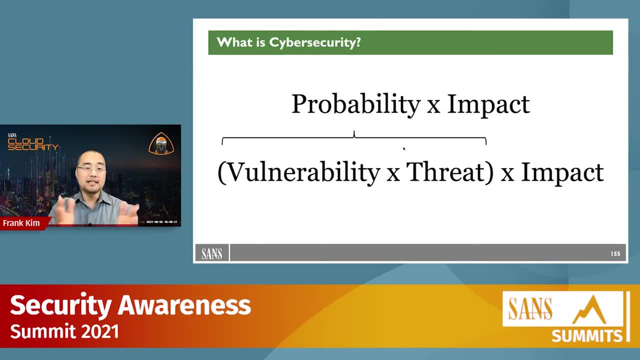 portion of the risk equation into two additional component parts: Vulnerability- what weaknesses, what misconfigurations, what issues do you have in your environment? times the threat, What are attackers, What are adversaries, What are threat groups actually doing? And it is a combination of 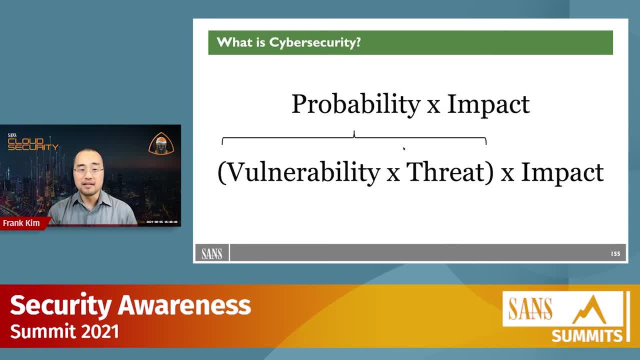 those two things that inform the probability portion of the risk equation. So we commonly say risk is probability of the risk to your organization overall. All right, Very important to make that distinction. Now security: so the cybersecurity industry traditionally, historically right, has 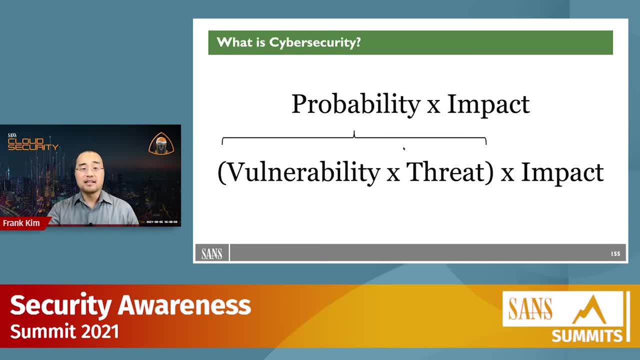 largely focused on the vulnerability component of the risk equation. How do we fix vulnerabilities, How do we prevent vulnerabilities, How do we patch them, And so on. And of course, though in recent times- right, not so recent times- the threat component has become the risk equation. So 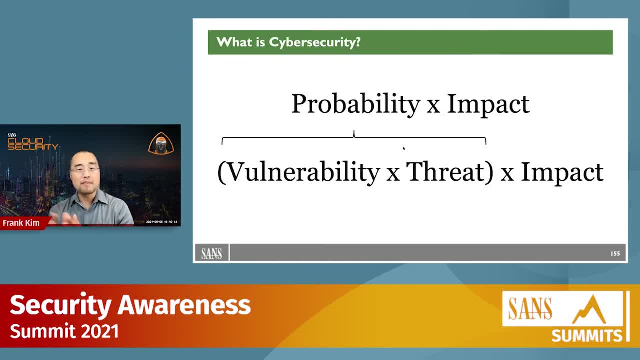 we've got frameworks, which we'll talk more about here in a little bit like a MITRE attack right. that has become the de facto standard for understanding what adversaries are actually doing. So there are good ways for us to understand and think about the probability here, But a lot of 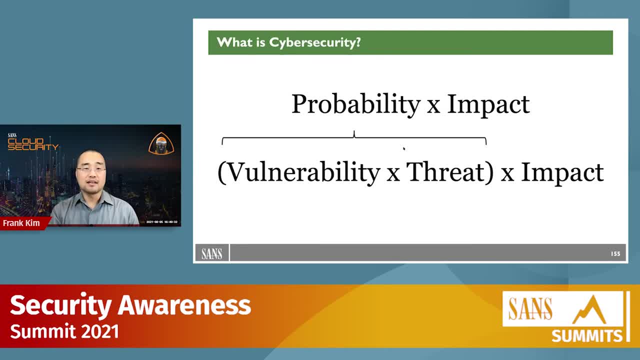 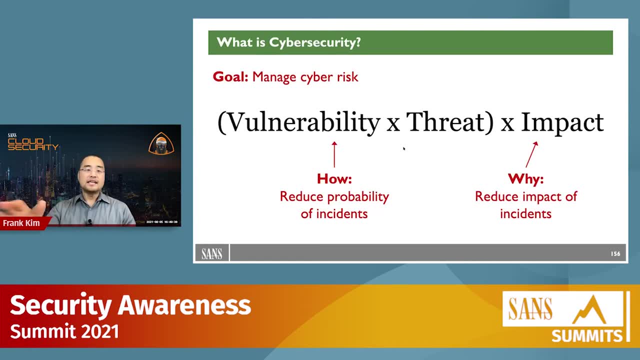 times, we in security, we don't necessarily have a good understanding of the impact, right? What's the corresponding impact to our organizations? Here, on the next slide, we're going to talk about risk, So let's go to the next slide, right? What is our overall goal? Our goal from a security 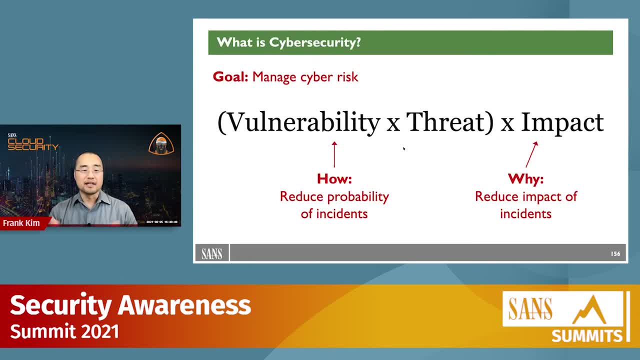 perspective is to manage cyber risk. Now, how do we go about doing this? Well, we do this by reducing, managing, mitigating the probability of incidents. And remember, when we say probability, we are talking about a combination of both vulnerability and threat. So this is why we 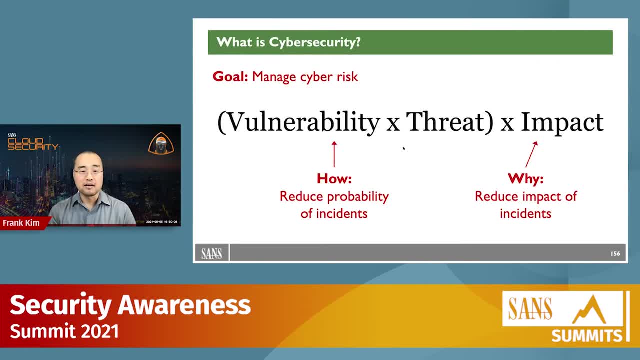 do things like: we install our firewalls, we install intrusion detection, prevention, we install endpoint detection and response, we take proactive controls to secure what we're doing on-premise and in the cloud, And now we factor in. well, what are the adversaries doing? 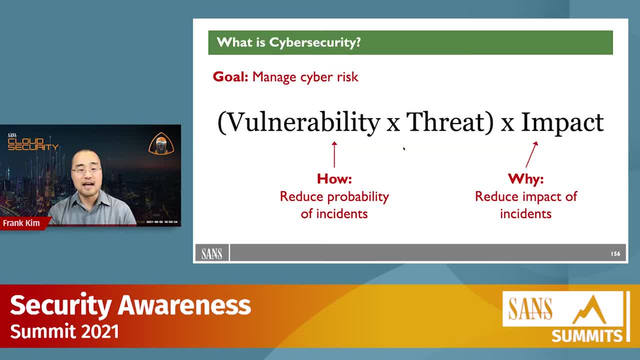 What are we doing to detect them? What are we doing to detect real attacker adversary activity? So a lot of times we in security we tend to focus on the how. What are the things that we do, that we need to do on a day-to-day basis? Extremely important: right Half of the overall. 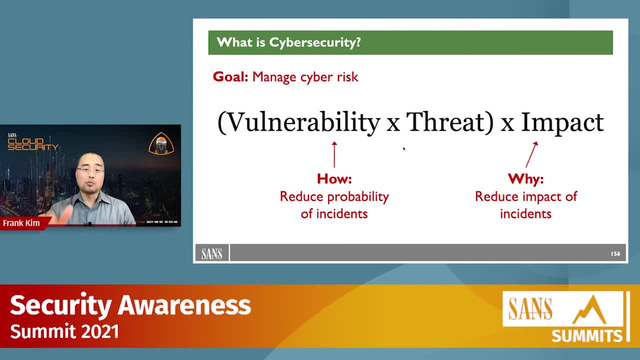 risk equation, But the impact. this is the. So why? Why do we do certain things? And we do it because we want to reduce the impact of our various security incidents. Now I see that David has a comment here that says: 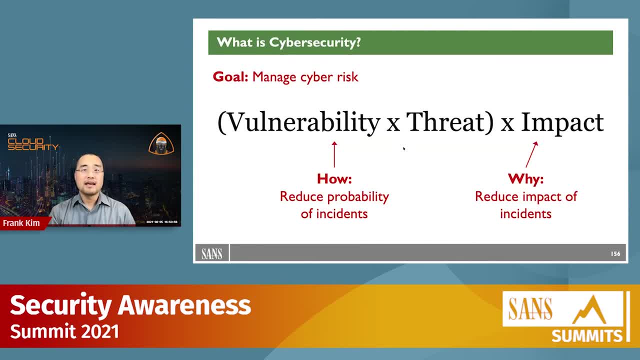 yes, of course, risk is impact times probability. But hey, you've read about some unknown unknowns, right Like the black swan events that have occurred, right Like, perhaps, the big financial crisis 2008,, 2009,, like the one that we all have just recently lived through and with. 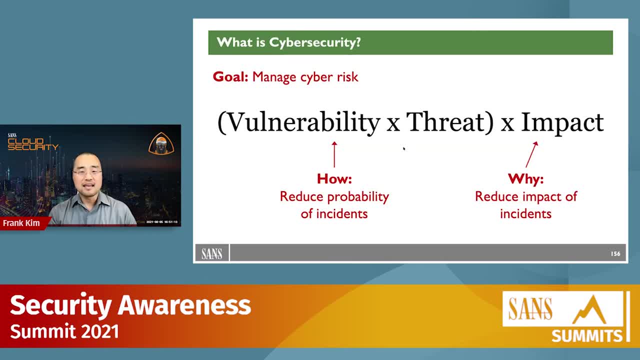 in terms of COVID-19.. Now you might look back at that and say, hey, you know, that was actually predictable, right, We could have foreseen that. In fact, various governments around the world had made plans, right Plans, to say, hey, there's the likelihood of the impact of an outbreak. 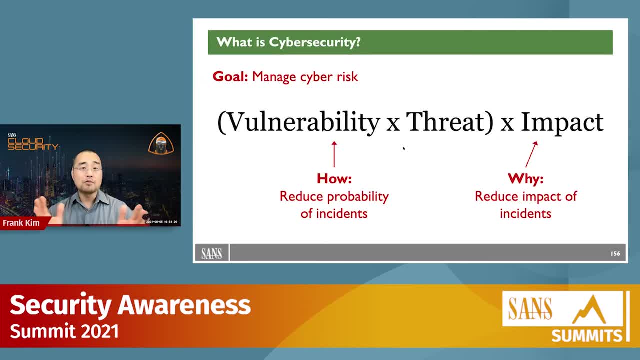 a global pandemic based on a new novel coronavirus. That would be pretty bad. However, a lot of organizations, a lot of countries, a lot of states around the world didn't heed that advice and take proactive measures. Well, they kind of had a sense, an understanding of the impact there. right, They didn't necessarily. 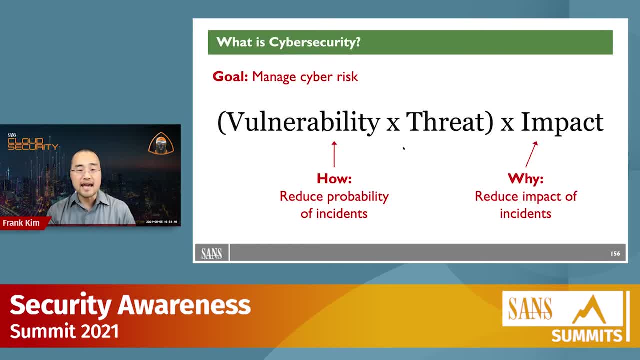 take into account. okay, well, how? What can we do today to mitigate the probability, the vulnerability and the corresponding threat axes? So yeah, David, I think I would still kind of incorporate that into the way that we look at risk overall. So if we're talking about 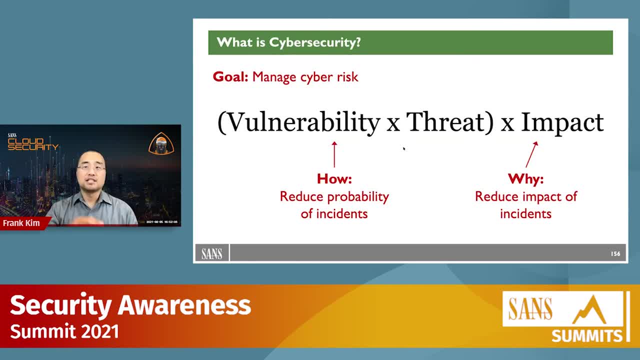 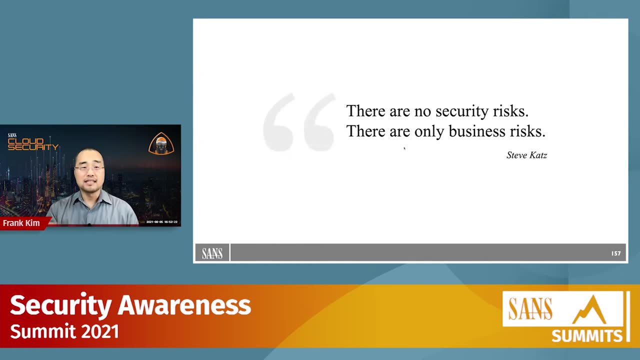 how do we go about managing, managing cyber risk? Well, that's our ultimate goal. Now, keep that mental. I'm going to mentally bookmark that for just a moment. in terms of managing cyber risk, I've got a friend, a mentor, Steve Katz, right. He's known as the world's first CISO. Maybe some of you guys. 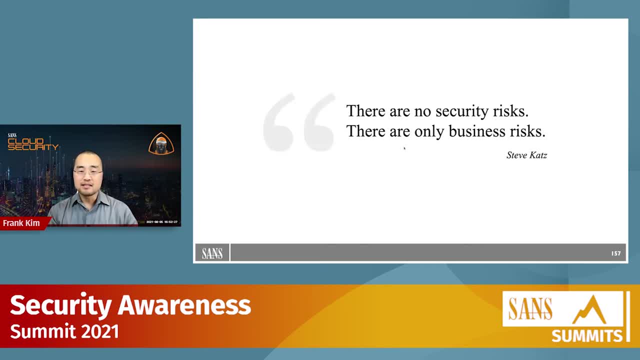 know him as well And I've heard him say this. He said this to me numerous times. He says, Frank, you know what? There are no security risks. right, It's not about cyber security, There are only business risks. And so I would definitely right what we're trying to talk about here and really 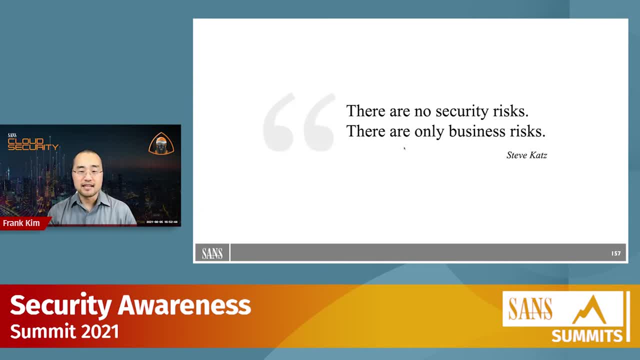 hammer home is that we want to be able to manage cyber risk. We want to be able to manage cyber risk. We want to make sure that you guys understand that, hey, we need to take a step back, as many other presenters have said, and understand. well, how does this relate to the? 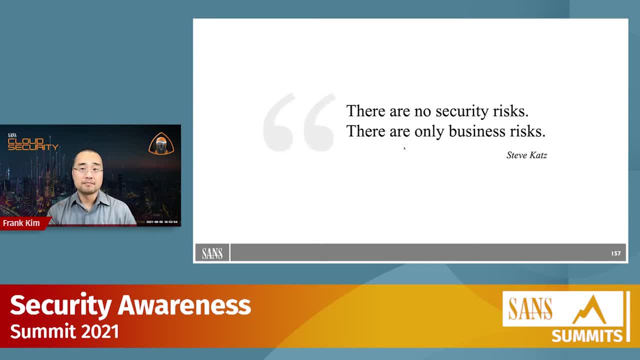 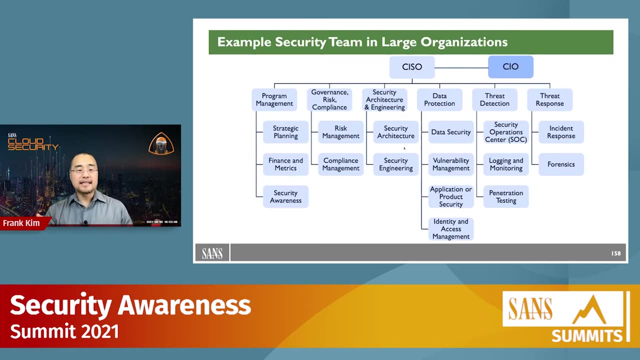 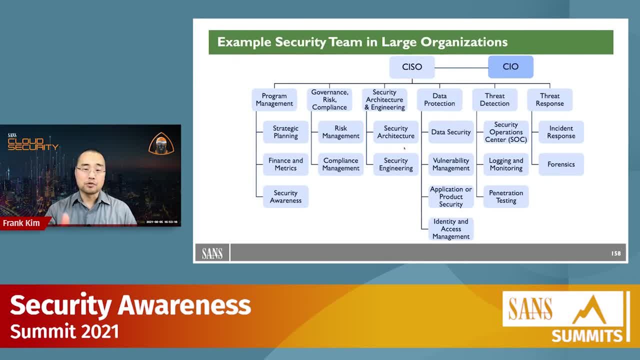 And this is, you know, still the majority of CISOs report up to the CIO. Now that is changing slowly, changing depending on the industry and depending on the company. Still, the vast majority of CISOs report within the technology organization And you can see here in this example, org chart. 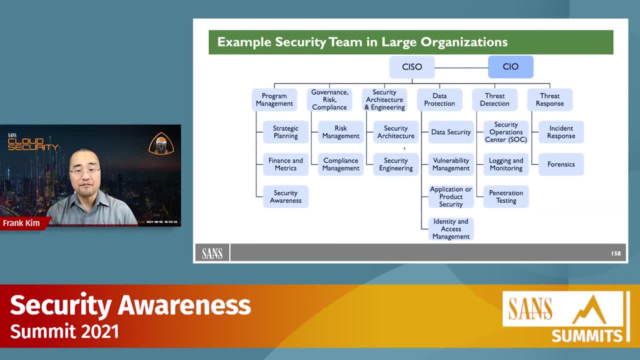 that there are various functions, activities that every single security team does, that actually tie back to that basic risk equation: doing things to manage and prevent and mitigate vulnerabilities, doing things to detect and analyze various threats. And well, there are certain things that we do to try to factor in the impact right. Why do we do these things from a business? 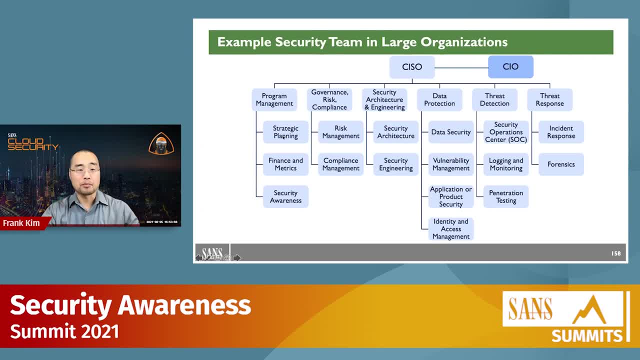 perspective, like governance, risk and compliance, like appropriate program management, strategic planning and so on. So Pauline has a perfect question here. She asks: hey, where would you position the security awareness program within information security, within IT compliance? 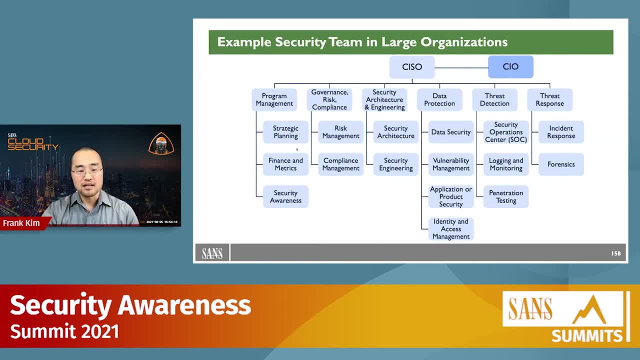 within risk management. Now in this example org chart- here you can see where it is And on this next slide right, security awareness. Well, what is it? Security awareness is just another control, one of the many controls in the cybersecurity portfolio here to control and manage human risk. 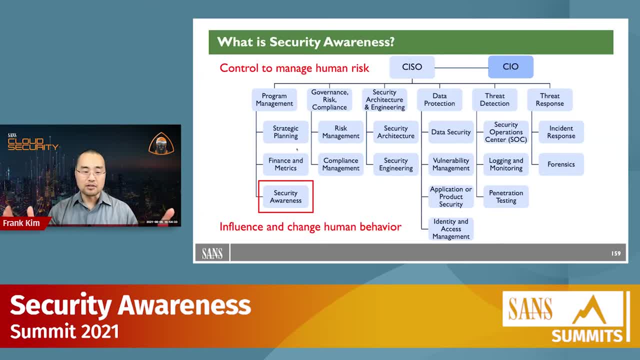 And ultimately, what is the goal of security awareness? Yeah, of course it is to influence and change human behavior, right? Because by influencing and changing human behavior we are able to control and manage human risk. And so, what is the goal of security awareness? 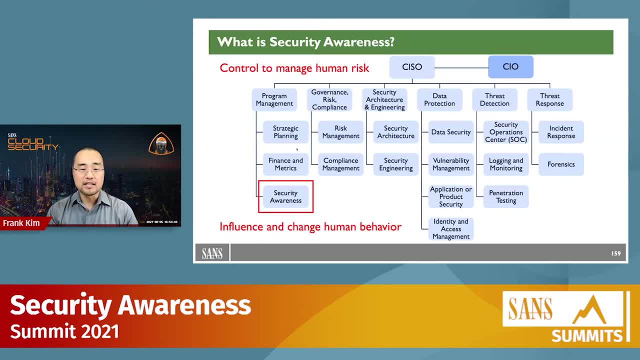 We are turning the dials on that risk equation overall. So specifically, you know, yes, I've seen security awareness many times live within the information security team And because of it being a key critical control right, which is generally where I've had it on the teams that 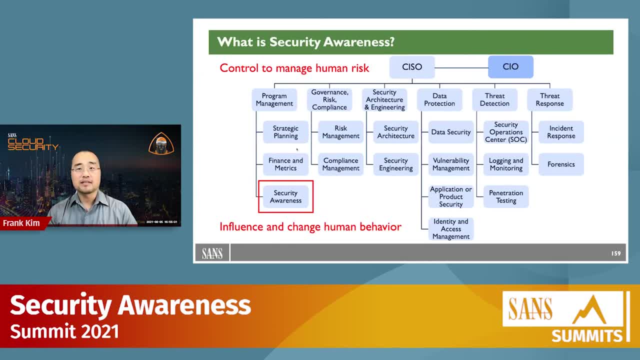 I've had in the past, but I have seen security awareness live in other areas, Pauline, as you're saying as well, whether that be in compliance, risk management and so on, But there needs to be a strong relationship in my opinion. And so what is the goal of security awareness? 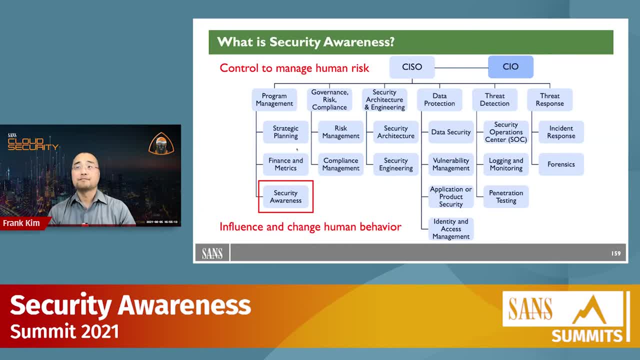 To the information security team, like we see here. So the question, the question then becomes: out of all of this stuff that you see here, all of the detailed things that need to be done by each of these teams, each of these boxes, how do we make a little bit more sense about it? You, as a 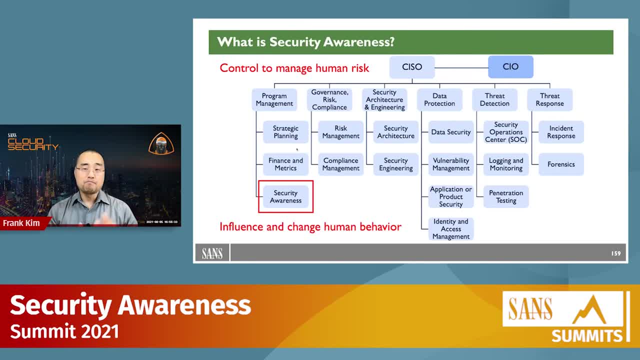 security leader. what do you need to do right to better frame, better structure this- the overall work of the security team. And what do you need to do to better frame the overall work of the security team? And what do you need to do, therefore, then, to better communicate and make 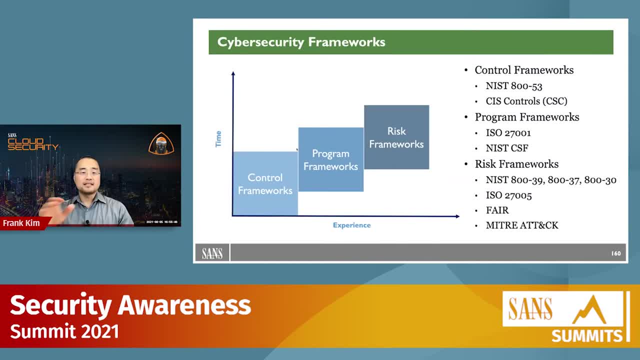 decisions about what actually needs to be done. Well, this here on the next slide, is where various cybersecurity frameworks come into play. Now, we're not going to go into all of the details of all of these frameworks- We don't have time for all of that- But I'm going to give a couple. 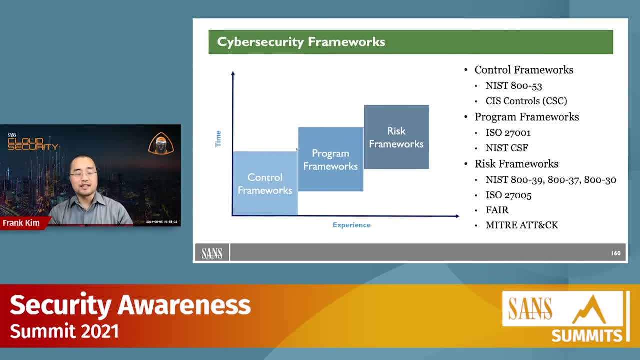 different examples here. right, We'll see a couple different examples momentarily. Now we know that in that org chart that we just saw, there's a lot of stuff that the security team does on a daily basis. There's a proverbial alphabet soup of complex things that tend to be. 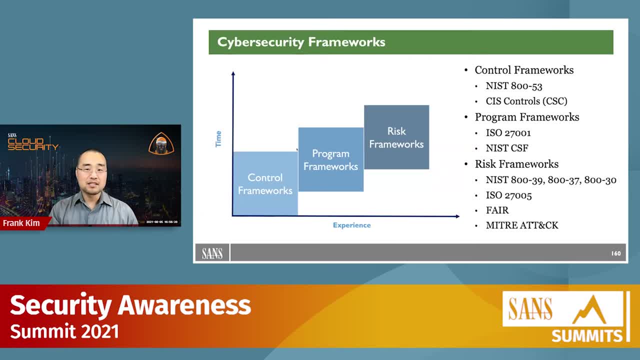 difficult for security people to explain. Lance mentions the curse of knowledge in another talk. that is happening And that's exactly what we're talking about here. You would think that security frameworks would be able to make the complex world of security a little bit more understandable. 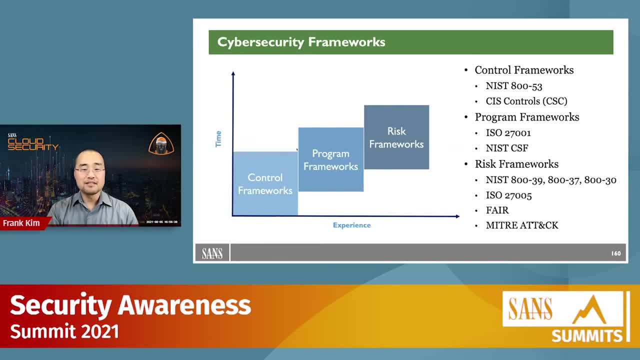 However, having read all of the details of these security frameworks, you would think that security frameworks. having, unfortunately, read all of the PDFs for the various things that we see here on the right-hand side of this slide, I can tell you firsthand that all of these frameworks- 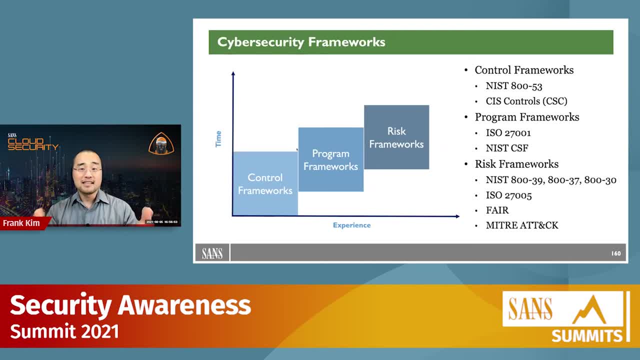 all of these documents don't make security less complex. It makes it even a little bit more complex. So how I like to think about this is: hey, there are three different types of security frameworks. Now let's draw an analogy here. Let's pretend that you want to be an amazing chef. 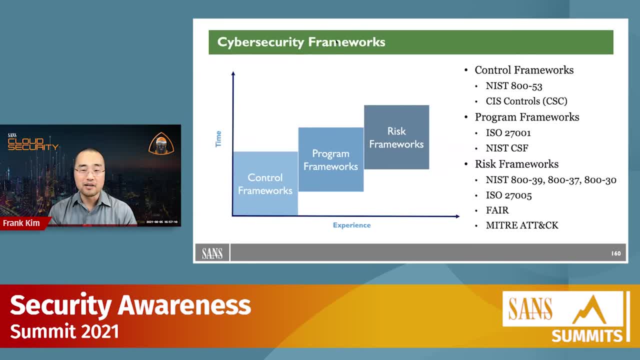 But unfortunately, like me- some of you may have heard me talk about this- unfortunately, like me, you're not a very good cook, but you have this dream, this vision: to become a world-class chef one day. Well, the first thing that you need to do is you need to know. 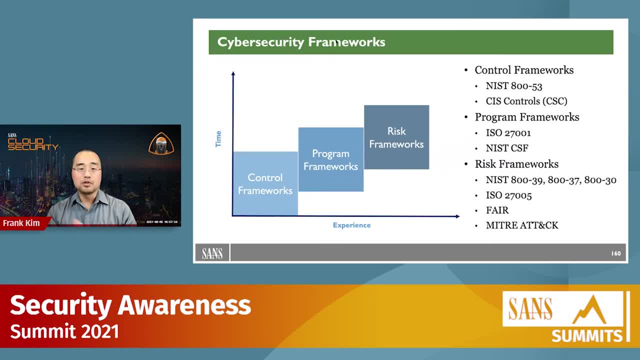 what ingredients are available to you, what works well with each other- garlic and basil, soy sauce and garlic and so on, whatever it might be. That list of ingredients is kind of like your control frameworks, right? What's every possible thing that you could put in the dish? 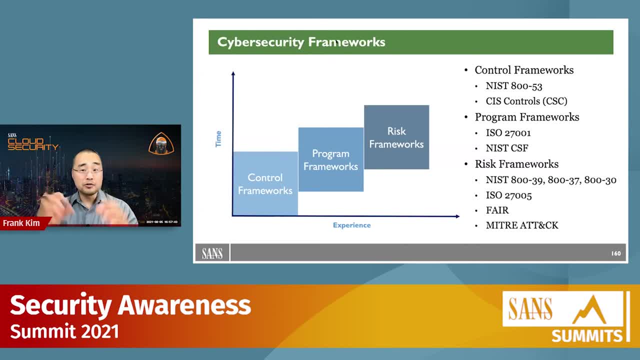 Well, you know that you can't make a successful meal by including every single ingredient, just like you can't create a successful security program by creating including every single security control. That's not going to work. So what do you do instead? You follow a recipe. 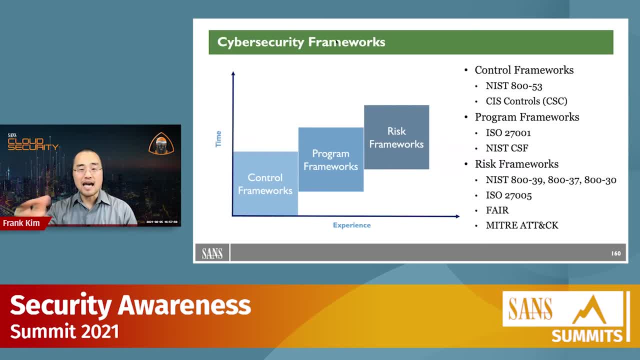 And the recipe defines: hey, what amount, what measurement, how much should you actually put in? That is the equivalent of your program frameworks there, right? What activities provide the most bang for the buck, What works well together, What will make the most sense, And so 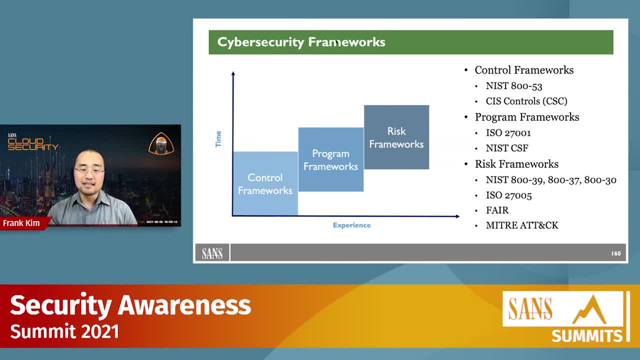 people like to taste, But it's not just about creating a delicious dish. If you want to become a world-class chef, well, you're going to probably have to open up a world-class restaurant. To open up a world-class restaurant, you need to know what do people value, right? What's the 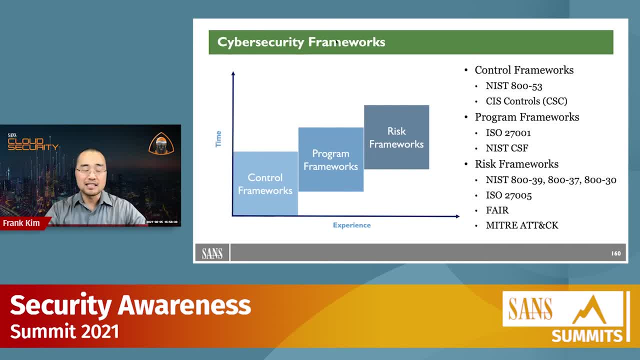 ambiance they're looking for. What's the vibe? Is it high-end, Is it accessible to more people? right, And you only know what people value, what the market values, what your stakeholders and customers value. if you understand, ah, you're going to be able to get that risk equation here. if you understand what the risk frameworks. 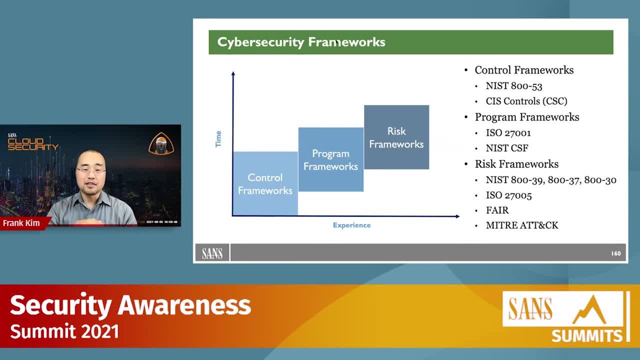 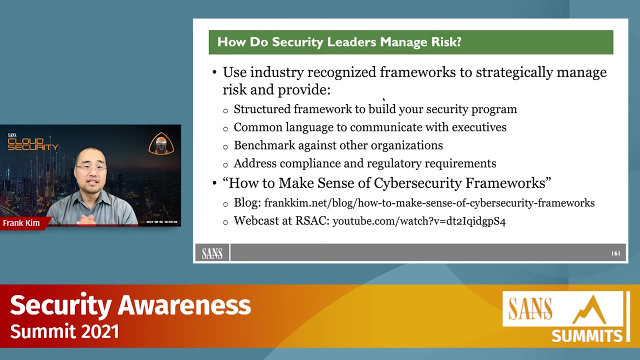 are What is the combination of vulnerability, threat and impact that you need to manage and present it in such a way that people will be able to understand. all right, So here on the next slide. how do you go about managing information, risk or managing ultimately? 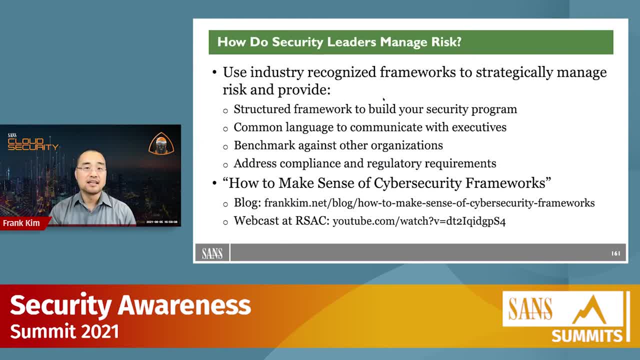 business risk- And I see Karen has this exact same question- is: how do you go about discussing right The need for all of these security controls versus the impact, the convenience, the availability, all of those different trade-offs? This is where the security frameworks come into play. 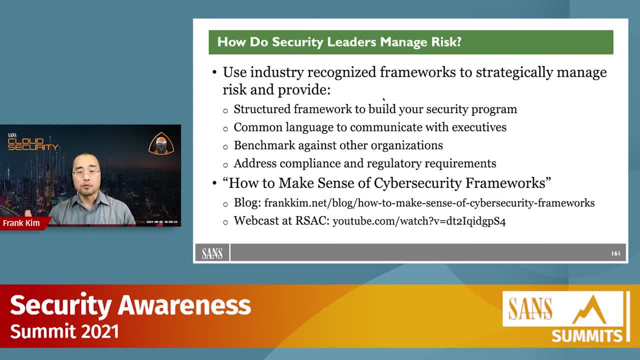 right At SANS. over the years SANS has done a lot of work talking to different board members, security leaders and so on, And board members unanimously say they say: look, we want you to give us some information related to industry standard frameworks and how we relate to others. 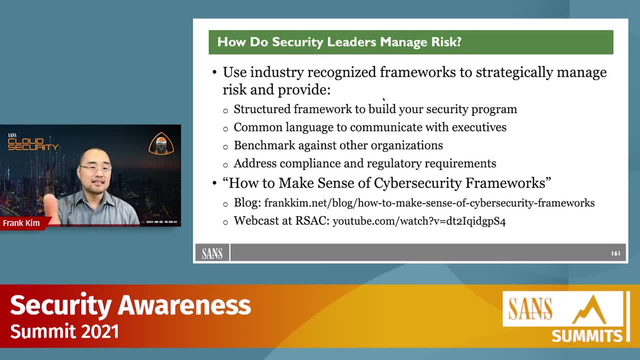 How do we compare to our industry? And this is why you want to use these industry standard frameworks: because: one, it provides you a third-party type of approach to structure your security program. It allows you to: two, communicate about that program in a consistent way And, number three, benchmark against other organizations. 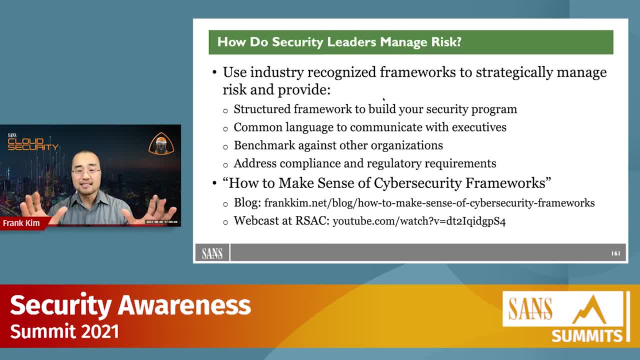 So if you are doing all of those things, you can then present that nice one-slide dashboard that says: hey, what's the comparison look like? And it's that type of thing that you're going to be talking about, And it's that type of thing that will inform your discussions with the business. 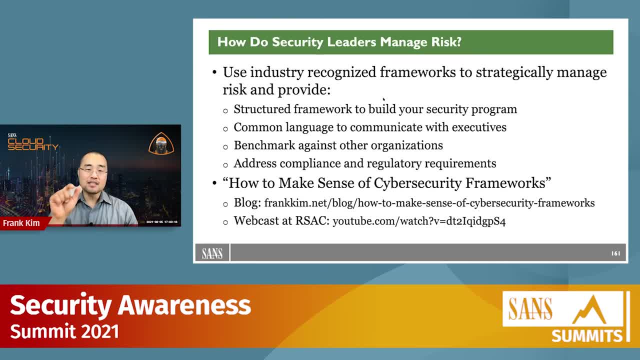 Because, remember we said cyber risk- They say, hey, if we turn the dial a little bit more here, right, will that allow us to go and do business in China and open up more markets? If we don't want to take that risk, well then could we turn the dial down so we don't have to spend and invest? 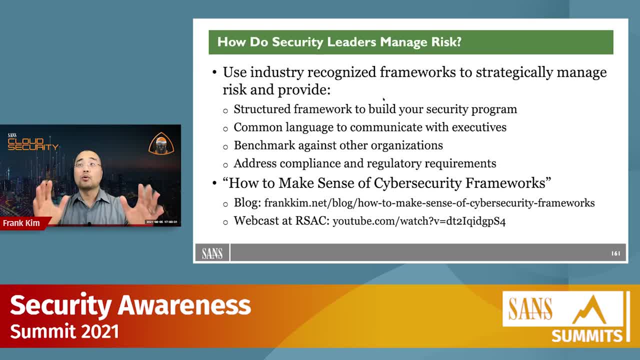 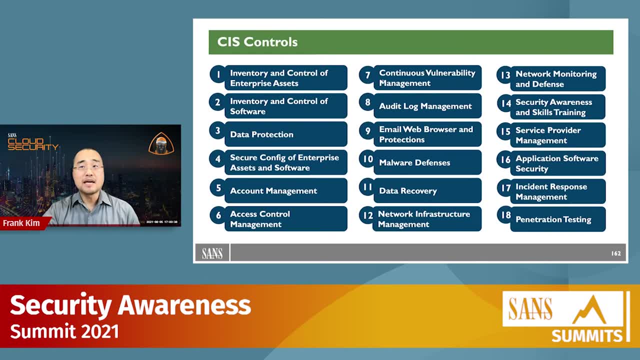 all of that money And it all comes back to what the organization's mission actually is. Now, here, on the next slide, let's go ahead and mention really quickly some examples. This is an example of one of the control frameworks We've got, the CIS Center for. 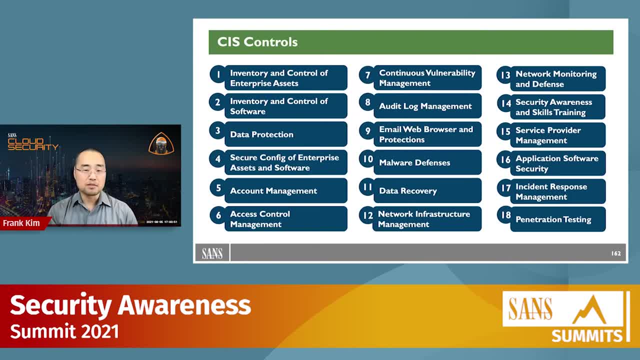 Internet Security Controls. The most recent version of this was just published a couple months ago or so, So I list this here as an example, Because if you just glance at this bunch of words here, you'll have a sense that these are the types of things that your security. 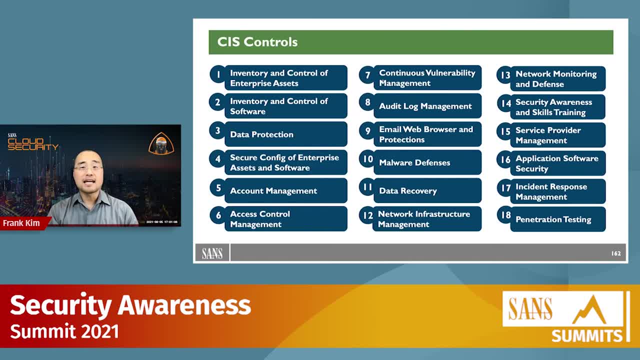 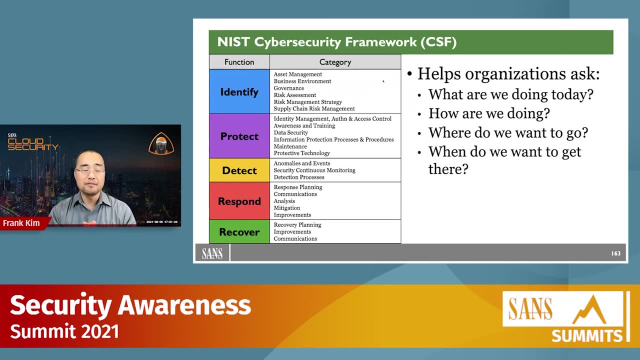 teams in that larger org chart. they're doing these types of things on a regular basis. All right, Now here on the next slide, we've also got an example of your program frameworks, And if I could actually switch to the next slide, there we go. The one that we'll mention here is: 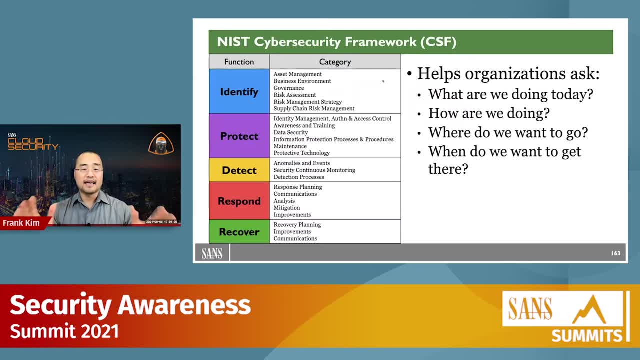 the NIST Cybersecurity Framework, CSF. Now I mentioned this one as a program framework, the recipe here that you might want to follow, because it is widely adopted, even internationally now, and it is well understood. Why do I think? 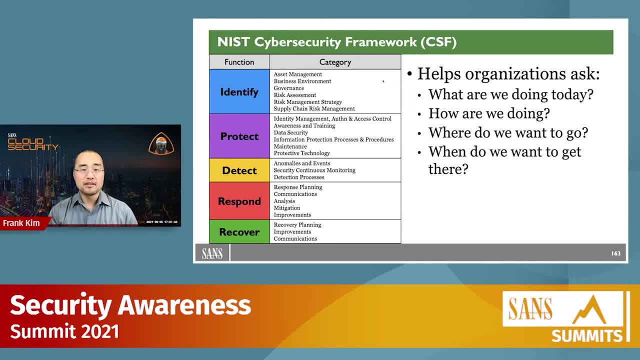 It is so well understood. Why do I suggest using that one? Because it is simple. Check it out. On the left-hand side is the core of the CSF, which many of you have probably seen before. This models the lifecycle of everything that every complex security team, every complex org chart actually. 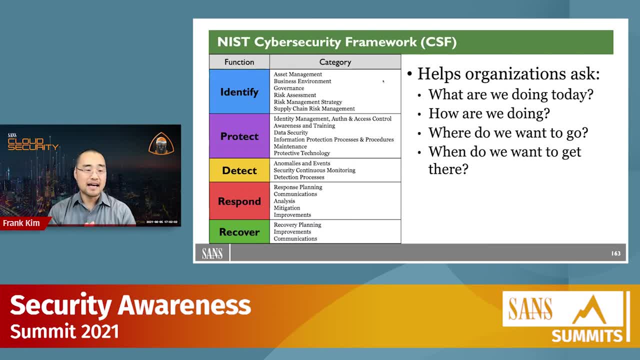 does We identify what we need to do. We identify our assets, our requirements. We protect, prevent bad things from happening If something gets by our protective capabilities, we detect them And then we respond to any of those things And ultimately we recover. Now David has a question. here is: 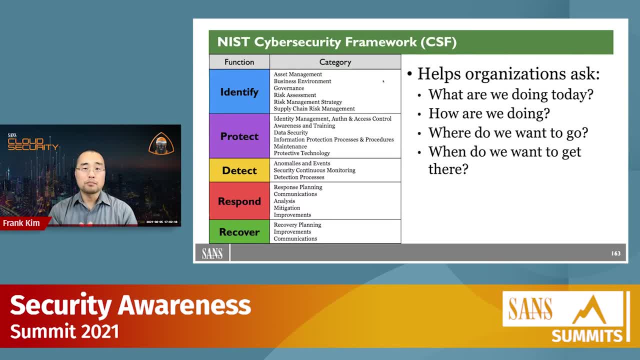 hey, where do you put side channel attacks in the control program or risk frameworks? Right, That's a very good question And you might have seen this on that slide where I had the three, I mentioned MITRE ATT&CK verbally. MITRE ATT&CK was mentioned on that slide. I put MITRE ATT&CK in the risk. 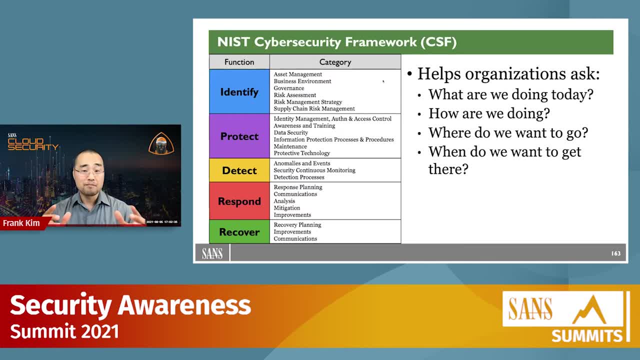 framework category for me specifically, because remember what did we say: risk is, Risk, is vulnerability times threat, And risk is vulnerability times threat And risk is vulnerability times threat. Where does threat go? Now, you could call MITRE ATT&CK a threat framework and whatever you might call it, But for us, in our business, 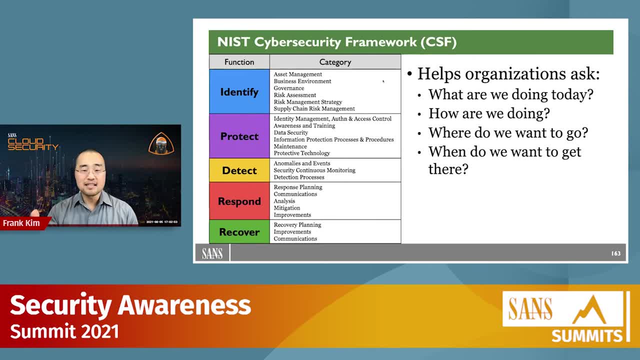 conversation. that category falls under the risk umbrella, right there. So that's how I would think about it, Because ultimately- remember, as Steve said, there are no security risks. There are only business risks here. Now Tina has another excellent question that is related to what we see here on the slide is: what are we doing today? 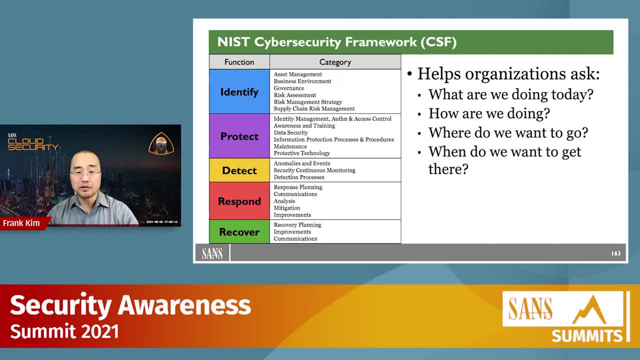 how are we doing this comparison to your peer groups and where do we want to go? Tina asks: well, where do you get information on benchmarking? Well, you can get information on benchmarking from some industry associations, groups that you might be a part of, like the. 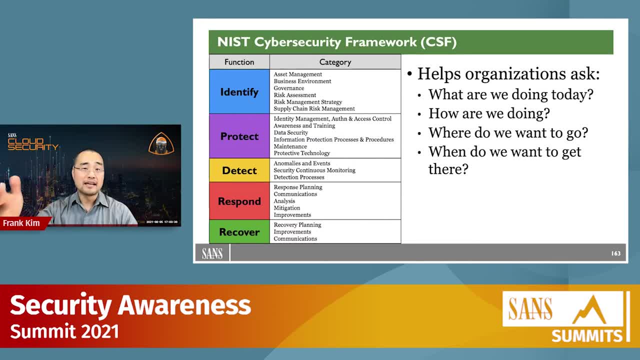 ISACs, the Information Sharing and Analysis Centers. whether you're in financial services, the FS-ISAC, whether you're in healthcare- HISAC, whether you're in an educational institution, the REN-ISAC, for example. So definitely there's some information sharing. that goes on. There's some. 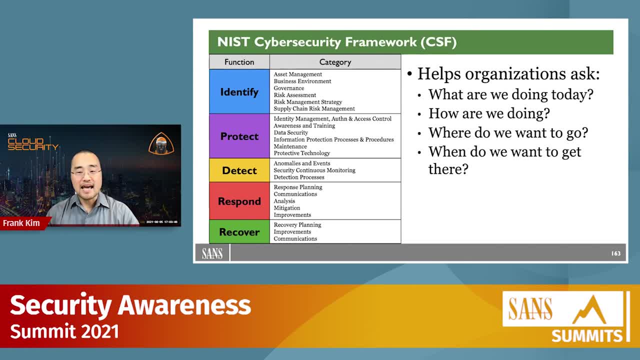 limited amount of that type of data that is available publicly. But also- yes, Tina, truth be told, where do you get that information? Generally, you've got to buy it from a consulting organization or from a research organization to get the most up-to-date data. All right, 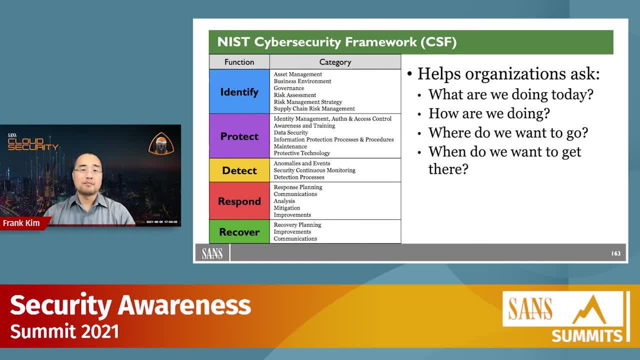 So Darren has another question here: Is there a framework for OT operational technology for ICS? Yeah, Yeah, there is. There's also frameworks like the C2M2 that was originally created by the Department of Energy That has since been made into a more broader framework. that's applicable. 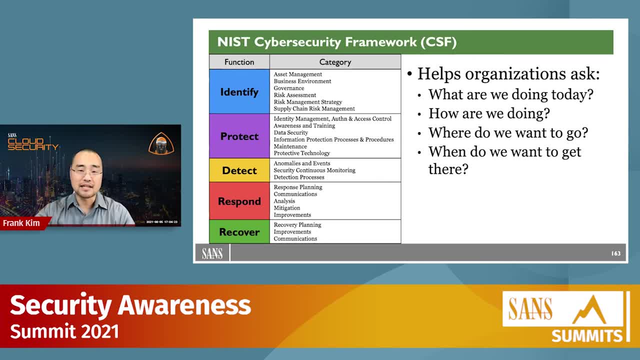 outside of just kind of the energy and the industrial control sector as well. So there's a number of ones that are available. I'm only giving you kind of a taste of what the many different frameworks that are available on the market are. All right, So now if we pause for a 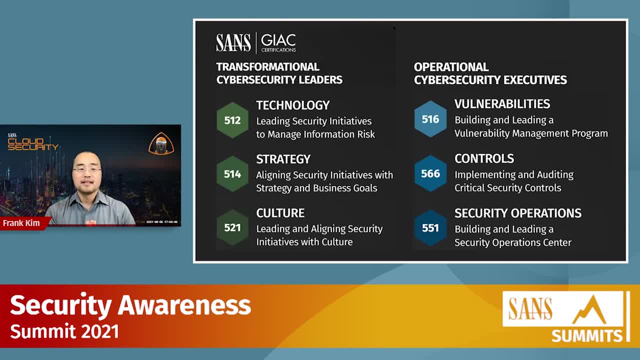 moment. All right, Let's take a step back, Right? Hey, we've been talking about what is the basic risk equation? Right? Why is that important? How does that tie back to the impact, what the organization is trying to achieve overall? Right, The why that we're doing these things. And then we talked about 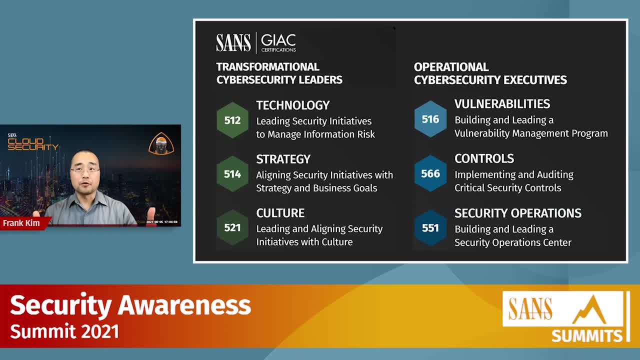 OK, how do we as the security team, how do we move those things forward? We saw where security awareness was one key, important control, But out of the many controls in the overall security portfolio. we saw where security awareness was one key, important control, But out of the many 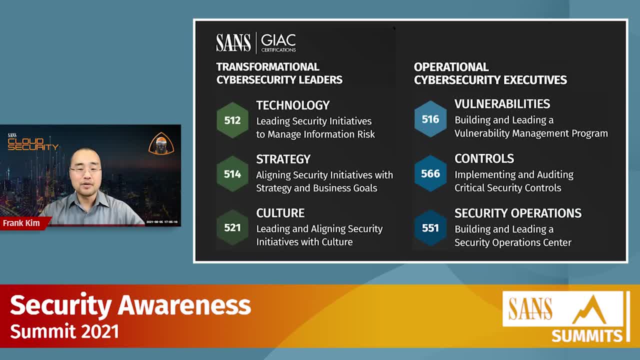 controls. in the overall security portfolio, we saw where security awareness was one key, important, and then we associate that with the different frameworks that we can use to better understand what we're doing. So for you, the security professional, as as you are progressing in your 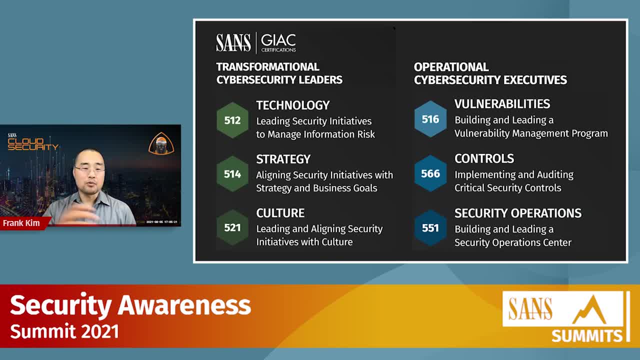 career. well, you want to improve, You want to get better, You want to make your organizations better. So how do we do that? Well, we found that, hey, to be a transformational security leader, to be an operational security executive. There are six key areas that you want to think. 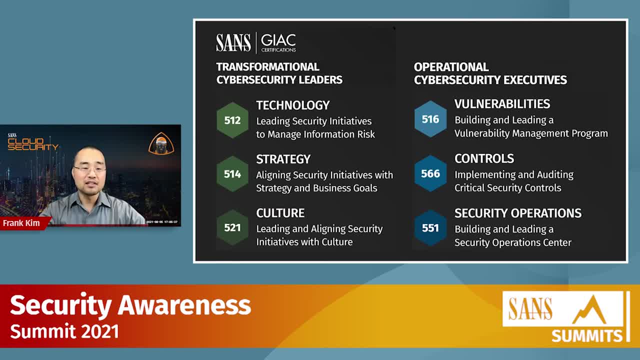 about. One is technology, but not technology for technology sake. technology for better managing information risk. The whole reason that we implement all of these controls, like awareness, is to better manage information risk. There is vulnerabilities, right, The corresponding vulnerabilities that come up, corresponding controls that could be. 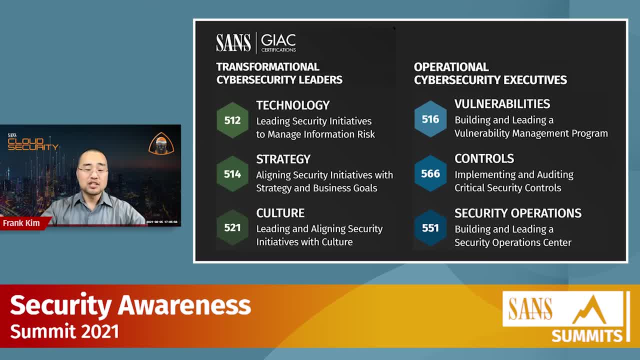 implemented to manage in the lower right-hand corner from an operational perspective, building out your SOC, your response, your detection capabilities. But there's a couple other key elements in the lower left-hand corner. right You've got strategy And this is about aligning. 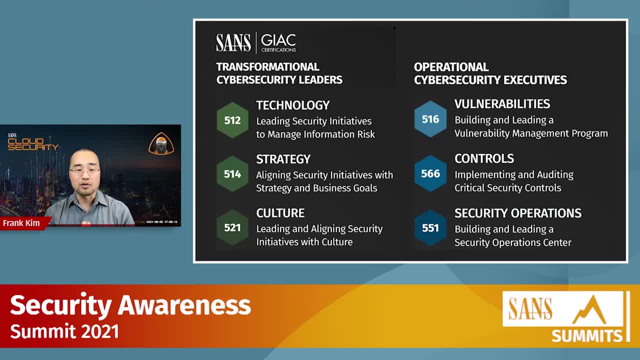 your security initiatives, All of the stuff that we saw on the org chart. you've got to make sure that those are aligned with your overall strategy, with your business goals. You've got to build a security plan that maps back to your overall business goals. You've got to build a corresponding 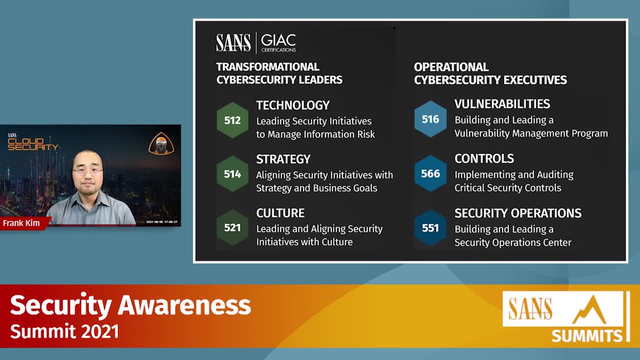 roadmap that will get you there. And oh, by the way, along the way you've got to make sure that your team and your organization builds those in in a sustainable, sustainable fashion. You've got to lead change, build a self-sustaining culture that will enable 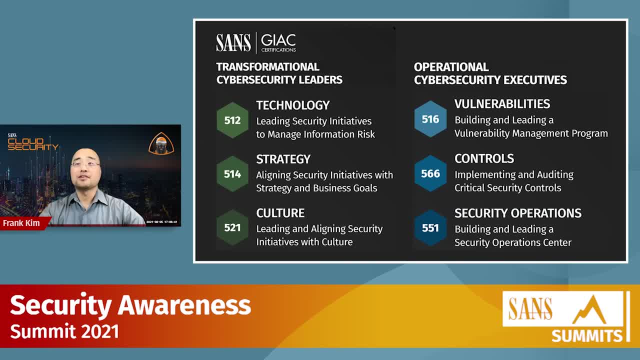 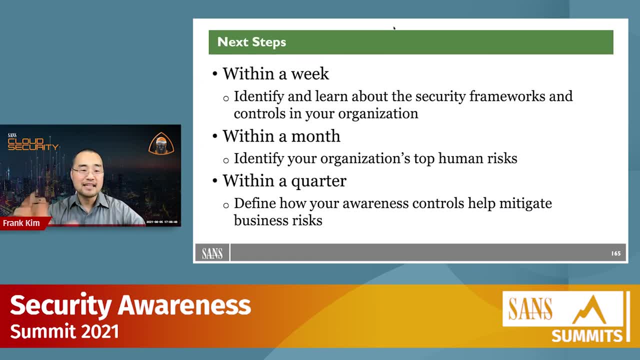 all of these things to continue on long after you're gone. So just to kind of summarize, what should you do? right Suggestion Next week? right, Go back to work And if you don't know already, go back and talk to some of your friends in the security team and say hey, 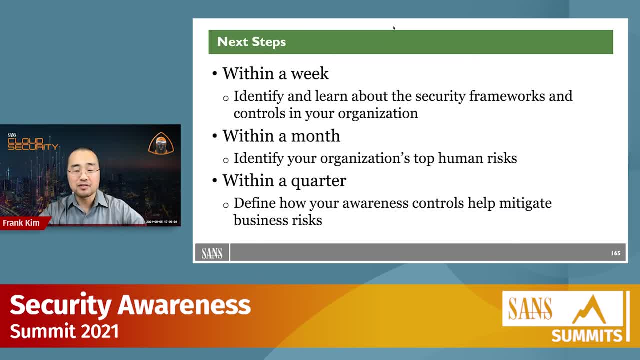 how did we structure our work? How did we structure our program? What frameworks, what controls are we using in the organization? Within the next month, think about what your top human risks are and then map those back to the controls right And see where there's some gaps or where there aren't some gaps or where. 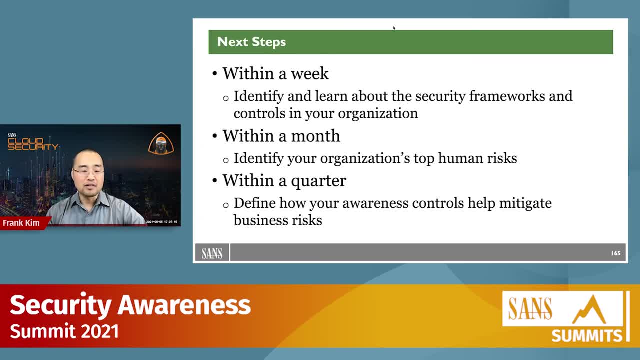 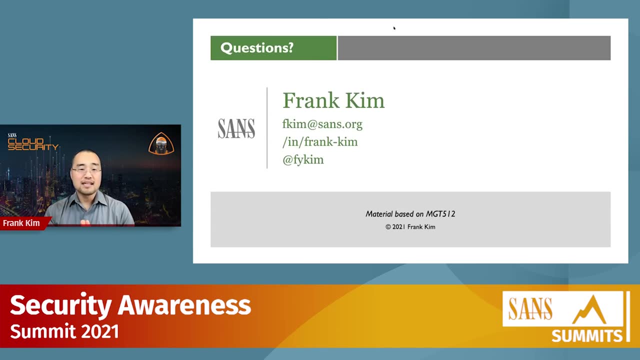 you've got coverage And then, with the next quarter and onward, go ahead and think about what are your awareness controls that will help you mitigate your overall business risks right? So with that, I'm going to go ahead and pause, close this out here. This was understanding. 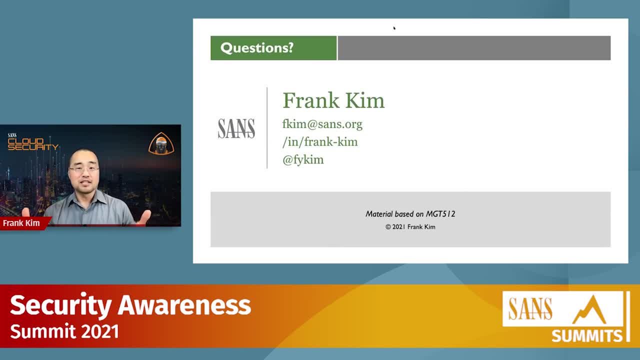 cybersecurity risk management really a an introduction here to remind ourselves of some of these common concepts, how it applies to the security program overall, how it's related to awareness, And with that I'm going to turn it back over to Lance. If you guys have any questions, want to stay in touch, feel free to reach out. 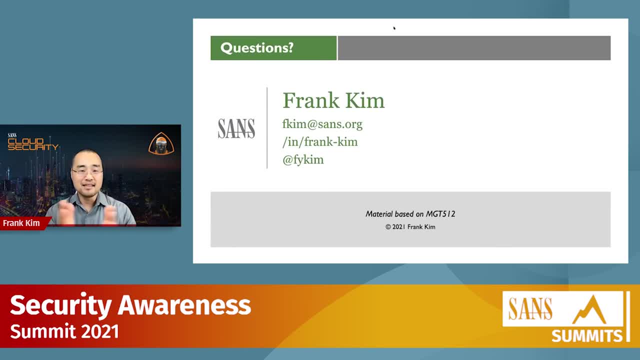 connect with me on LinkedIn. shoot me a note whenever you like. Lance back over to you, All right, Frank. Hey, thank you so much. Just to follow up to Frank's point. First of all, I know sometimes this may not be the most riveting, but this is what makes the difference. 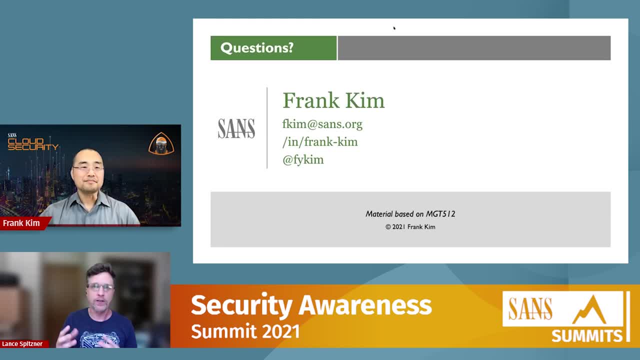 Between just being in the entertainment business and being in the human risk business. So if you weren't some of it you know you weren't sure about, please reach out to Frank. He's here to help you. We actually covered a lot of very serious concepts here in this overview. Now Frank, 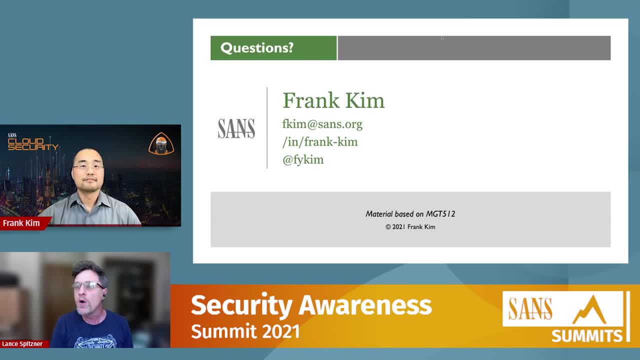 there's one or two questions, but I just wanted to follow up with Pauline who asked: you know, where should security awareness fall under? And I just wanted to follow up to Frank's point. You want to be sure it's aligned with and preferred. 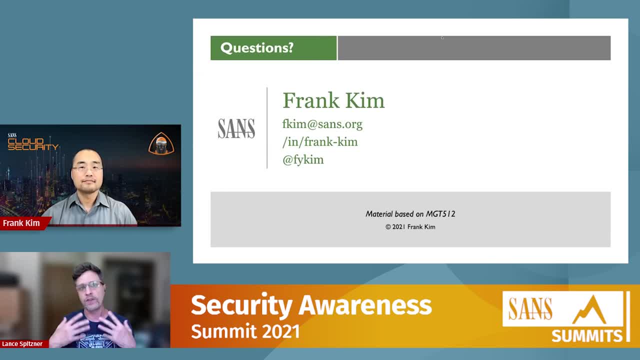 preferably under security. What we tend to find is, if security awareness falls under human resources, compliance or legal, it tends to take a very much compliance or legal focus, So you tend to be stuck in stage two, compliance of the awareness program. Remember, we're very much. 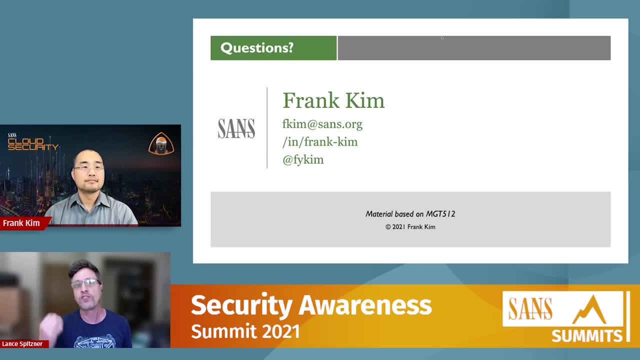 focused on. we want to enable you to have an impact, change behavior, manage human risk, And to do that, the closer you are aligned with the security team, the more you're working with them, the better. That's why I was so excited to see Frank make that. 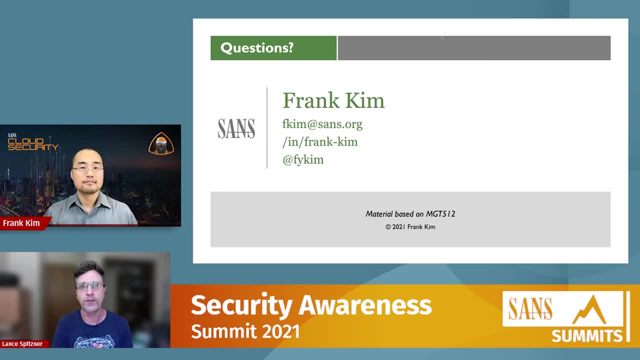 recommendation, Your very first step: go back to your security team and ask: hey, what frameworks are we using, What are our key controls And how can I better align what I'm doing with those frameworks and controls? Because if you are aligned with your security team, you now get more. 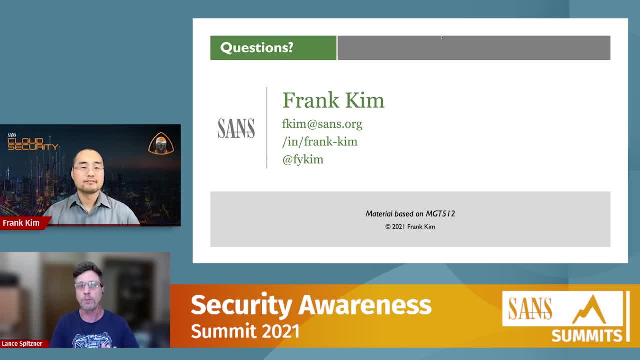 credibility, visibility and support, because you're supporting the overall strategic mission of managing Risk. Let's see here. Tina had a question, Frank, I'm not sure if you answered this one. Do you have any recommendations of peer groups or frameworks that focus on benchmarking? 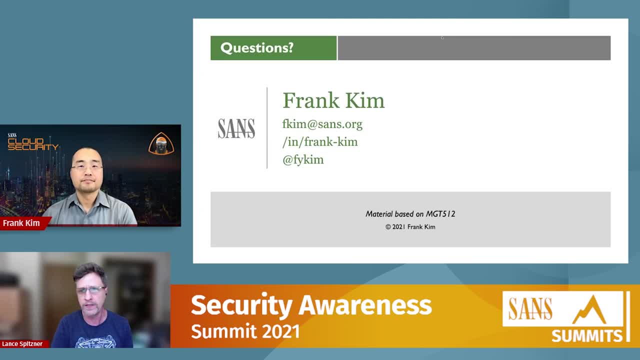 cybersecurity risk And I believe you answered that one. Yeah, yeah, We talked about that. But now that you highlighted this, I see another kind of related question here from David related to talking about business risk and the reason to benchmark, see how we're doing compared to others and ultimately to manage our business risk. 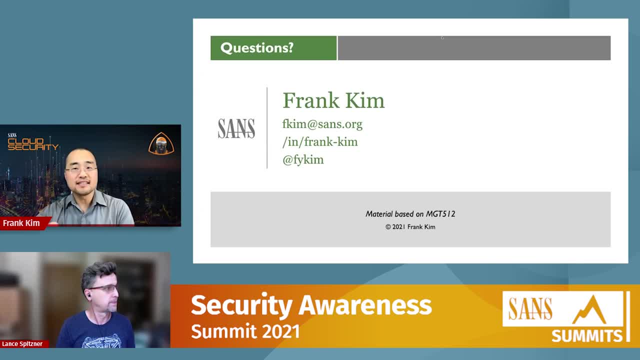 But David also asks: hey, are there some weak signals in the frameworks Or are there other tools? How do you understand what the business risk actually is? And this is one that I would recommend where? hey, when you're going back and you're talking to your security team. 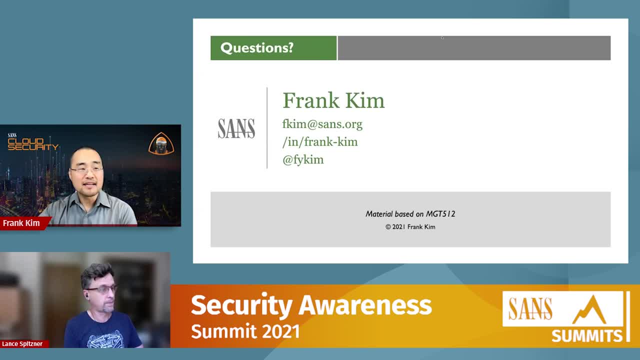 what controls, what frameworks are using. in parallel, go back and set up some meetings with some people that are outside of IT, outside of security, some of the business unit leaders, and just try to get a better understanding of what the business is doing, how it makes money. 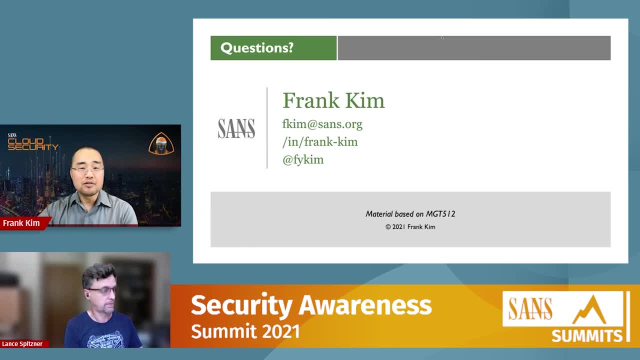 If you're a publicly traded company, go ahead and download the quarterly reports, And there's a lot of information there in terms of how the business actually works, what the different business lines do, And because if you don't know about that stuff, how are you ever going to have a conversation?